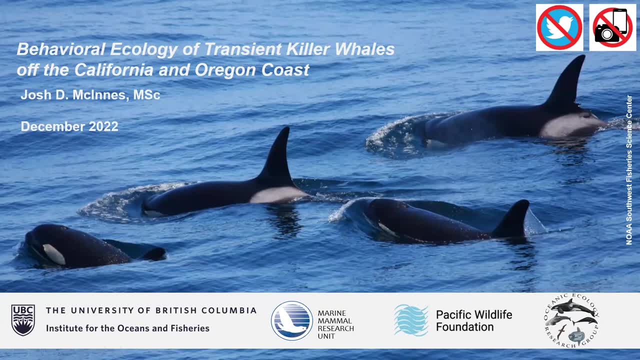 I just wanted to say thank you to Cape Perpetua for having me today. I'm pretty excited about speaking about killer whales along the Oregon coast in California, about their behavior with ecology. I know it's been kind of a new topic for the last couple of years as a lot of people are starting to see more and more killer whales and we were very excited as our research team has been working hard with the Oregon community to try to better understand them. 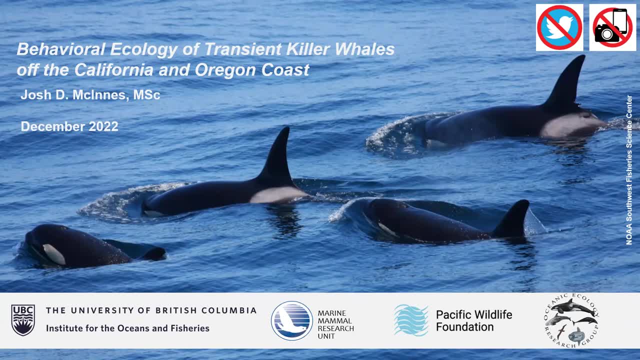 So, as mentioned, I'm a research scientist with the University of British Columbia's Institute for Oceans and Fisheries, the Marine Mammal Research Unit, but I'm also a research associate with Pacific Wildlife Foundation and as well as a leader with lead research with the Oceanic Ecology Research Group. 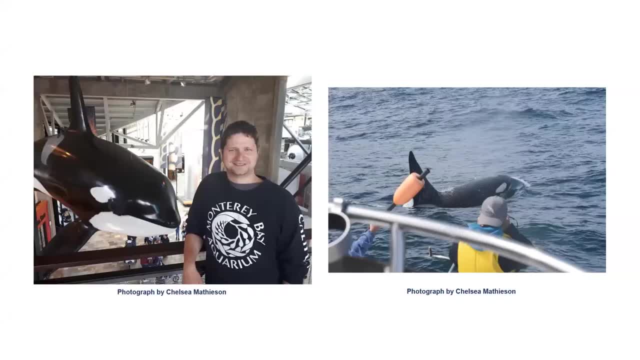 So just a little background. I spent since early 2000s working with killer whales. In particular, I grew up on southern Vancouver Island where I spent most of my time in Puget Sound area as well as the Salish Sea, working on trying to better understand the transient mammal eating killer whale form, which I'll talk a little bit more about. But I also studied resident killer whales and offshore killer whales and it's been kind of a life goal to kind of follow these animals and try to better understand them. 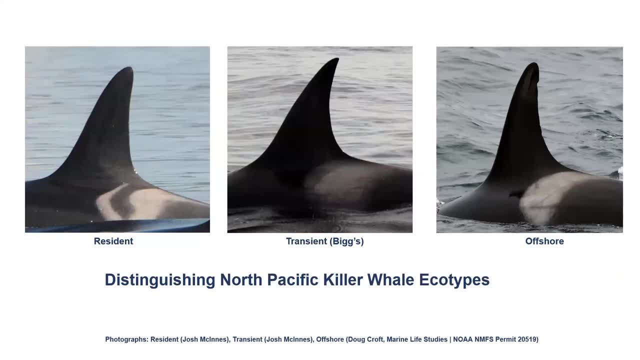 So just kind of a general overview. There's three ecotypes Now. an ecotype is a genetically distinct population, or basically it's a a. it's a fancy term scientists give to an animal that they really don't know what's going on. So one species of killer whale is known globally, but we have multiple populations that are kind of distinct. 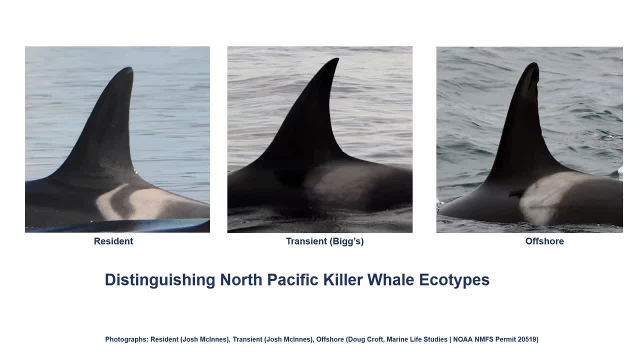 For instance, here we have three ecotypes in the northeastern Pacific that are all genetically distinct, as well as acoustically and even morphologically. So you can see, on the far left here this is a what we call the resident killer whale. 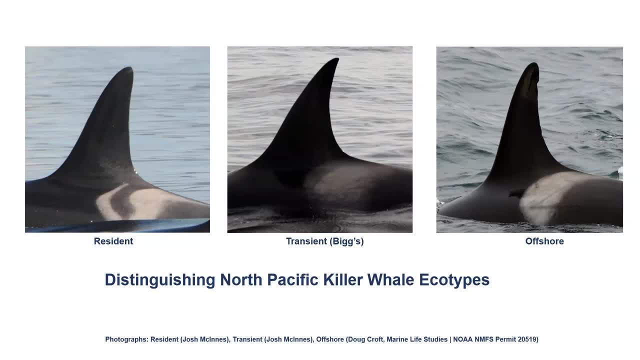 We know two different populations: a northern resident as well as a southern resident population. They predominantly eat killer whales. They also eat salmon, other fish species as well. They live in groups of between five to 50 animals. The killer whales are also based on this matrilineal system, where it's a female and her offspring. 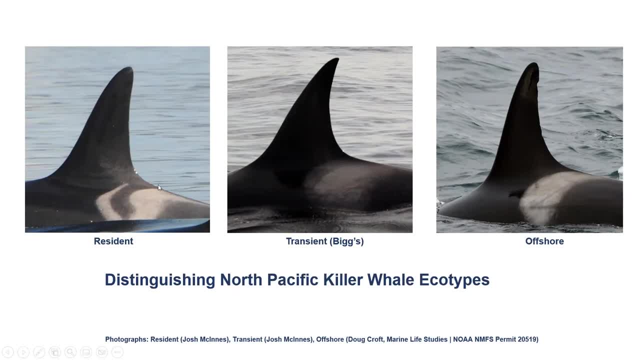 And resident killer whale society is really strong when it comes to that, that, that that, the matriarchal where there's no dispersal of male or female offspring. And we see these animals, particularly the northern resident killer whales, anywhere from the the northern resident killer whales to the northern resident killer whales. 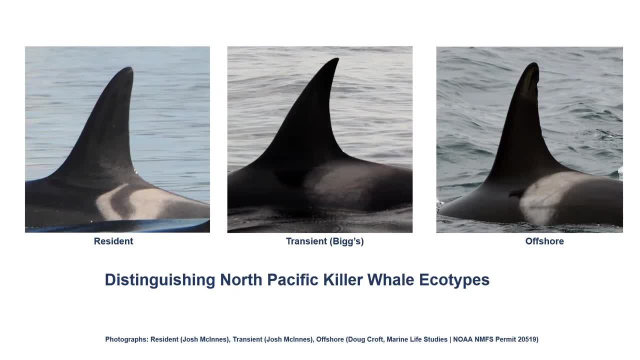 We also have the middle of Vancouver Island up to southeast Alaska, And then we also have the southern residents which we we see from basically the Salish Sea, southern Vancouver Island, southern British Columbia, all the way down to southern, down to central California. 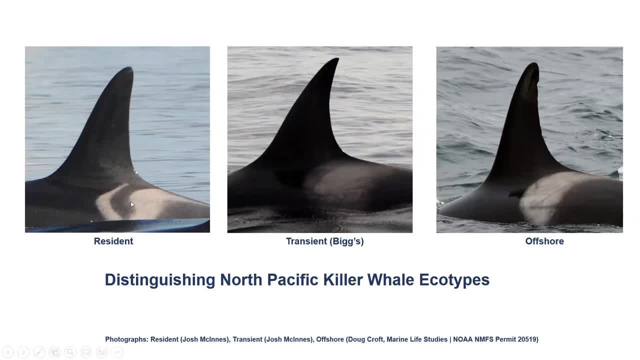 And off the Oregon coast we're starting to see more and more reports of southern residents, especially out in the fishing banks. Our research team has been picking up a lot of sightings of southern residents out there, and particularly one of the new calves in one of the three pods, K-pod. 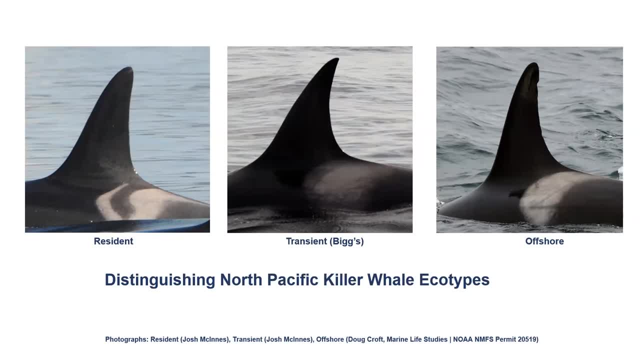 So there's J, K and L, Which are all part of the southern residents, and one new calf was actually identified off Oregon for the first time in the summer, which was pretty exciting. The population I really spend a lot of my time, though, is understanding is the transient. 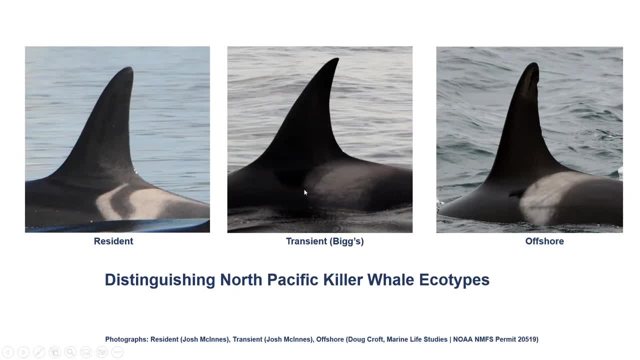 You can see here the way these animals look. the morphology is very different. Transients are kind of recognizable by seeing small groups. It can be a lone male that can be sighted, similar to if most of you know who T49C is. that might not ring a bell, but there's a male that seems to spend a lot of time. 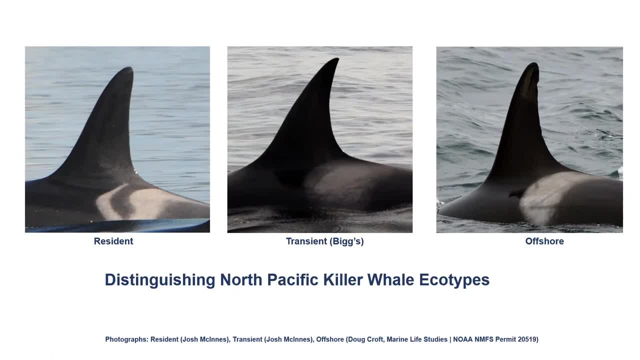 In around Coos Bay up in Tillamooka. he's always looking for seals. These guys are mammal hunting specialists, So they live in coordinated groups of between one animal, as mentioned, to up to 12. And they're very much on the lookout for anything warm-blooded. 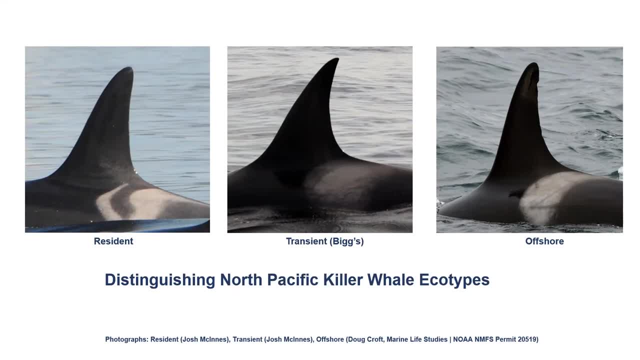 So that's seals, sea lions, porpoises and small whales, And then the last ecotype here that we have, which, if you're a tuna fisherman or if you're a fisherman working offshore, you might have an opportunity to see them. 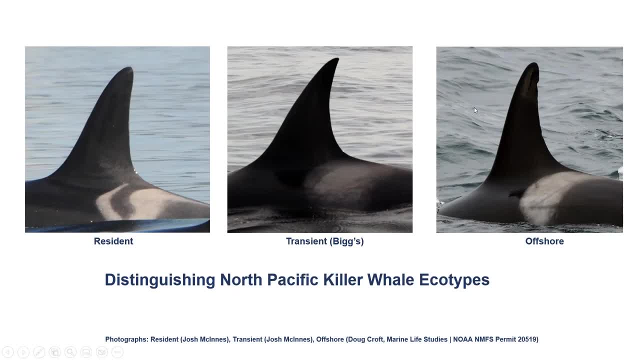 These are the offshore killer. These are the offshore killer whales which we don't really know a lot about them, but they form groups anywhere between 10 to over 100 animals And they're known to feed predominantly on fish species, but in particular, much higher trophic or higher food web species like sharks. 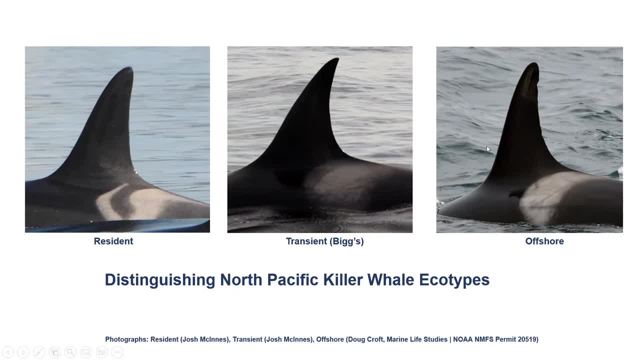 But what's the most interesting thing about these three populations is the differences in diet fish, telos species, marine mammals and larger fish species, But that they don't interact. They don't interbreed or mix. All three populations form their own communities that don't intermix or breed. 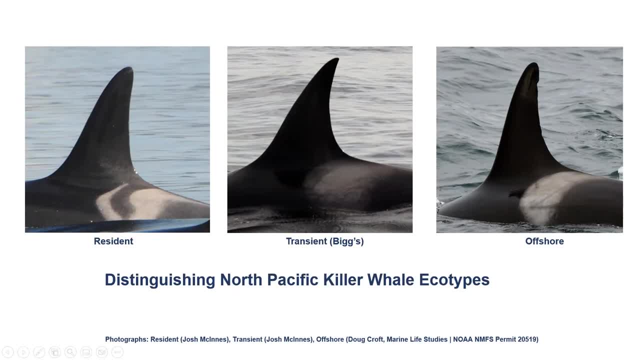 And you can see the differences based on the social isolation and reproductive isolation in their morphology. So resident killer whales are kind of recognized by this very rounded dorsal fin And this gray area called the saddle patch can be either open, with black pigments that kind of enter, or it can be closed where- and this is a closed saddle patch here in the transient, which is just all gray- 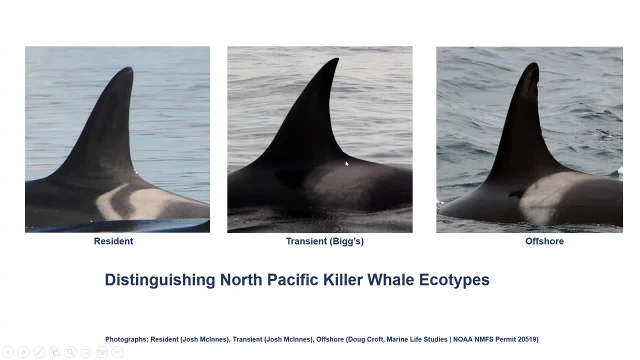 Transients, on the other hand, have a very pointed dorsal fin, typically very shark-like, and this is predominant in adult females- sometimes a bulge rate in the front area of the dorsal fin, but their saddle patches are always closed. We've never seen a transient killer whale with an open saddle patch. 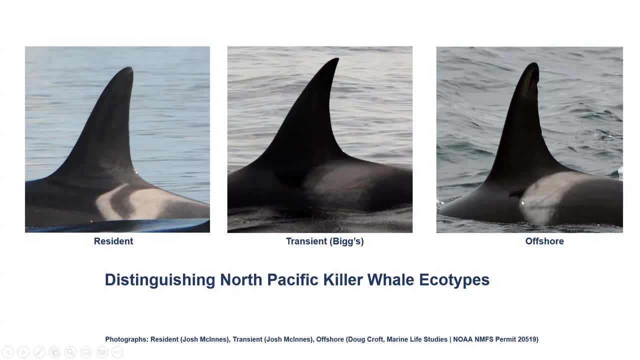 Offshores, though, are kind of a mix. Their body size in general is quite a bit smaller than the residents and transients, but they've been known to have either open saddle patches, similar to the residents, or closed saddle patches, similar to transients. 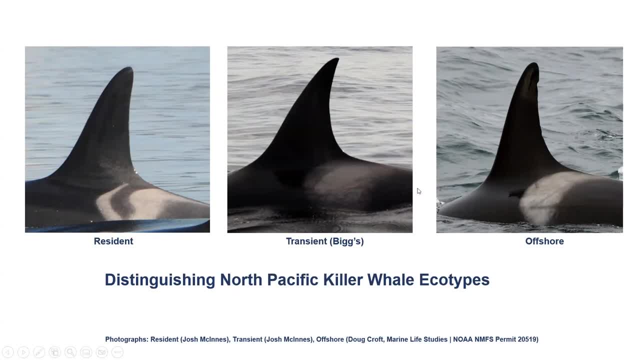 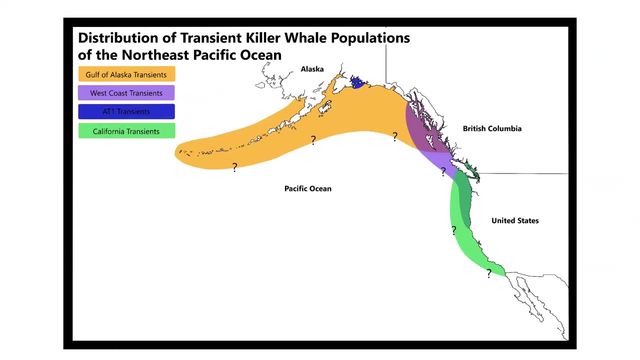 But all three are what we call sympatric, occurring in the same waters or the same ecosystem, but with a little bit of differences in where they seem to spend their time, depending on the prey species. But today I'm going to kind of focus on transient killer whales and I'm going to spend my time talking about two regions which our research team is very interested in, and that's the Oregon coast as well as the California coast. 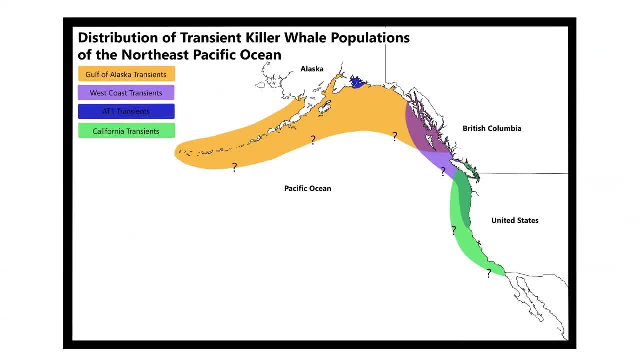 Two very productive areas, but transient killer whales are found pretty much throughout the northeastern Pacific, all the way from southern California, California, all the way up into the Bering Sea and around the Aleutian Islands in Alaska And, similar to the residents where you have a southern resident and a northern resident population, we have multiple populations of transient 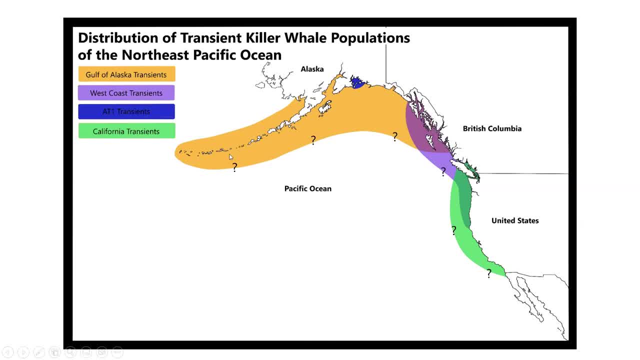 So, for instance, the Gulf of Alaska transients in the yellow here are a population that are predominantly seen throughout the Gulf of Alaska, in Prince William Sound, along the Aleutian Islands and into the Bering Sea, but also even down into northern British Columbia there's been a few sightings. 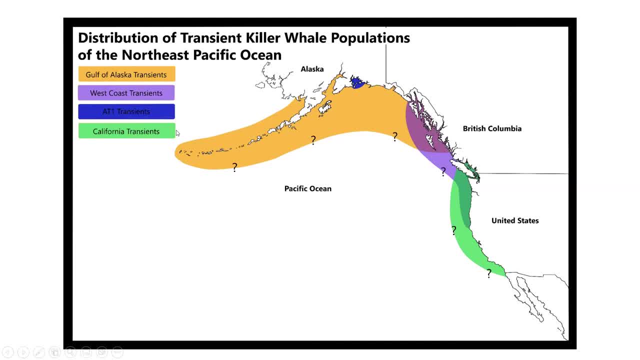 So all three, all these populations here Are genetically distinct as well as acoustically, and they don't intermix for the most part. This dark blue, this kind of blue AT1 transients, and this little dot right here is a very unique population that was discovered in 1984. 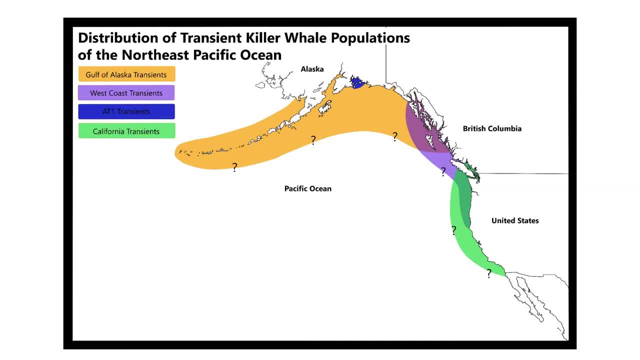 The AT1 transients, or whether we also call them the Chugash transients, are only found in Prince William Sound, And in 1984, when discovered, they numbered 22 whales, But after the Exxon Valdez Oil spill their population dropped to 13.. 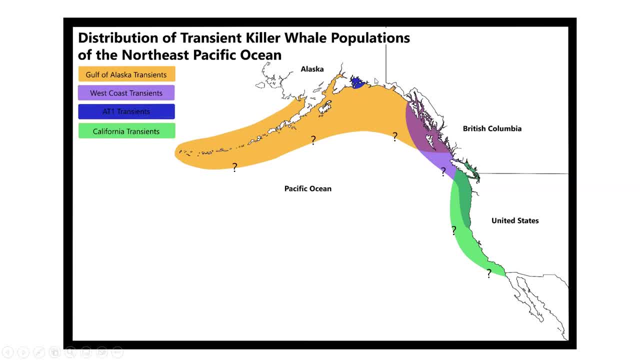 And now they're down to seven with no reproductive female. so that population right now is critically depleted under the Endangered Species Act and will likely go extinct. The other populations that we have, the one that's the best or the most well known population that occurs along the Oregon coast in California is what we call the West Coast transients in the purple. here in the green. 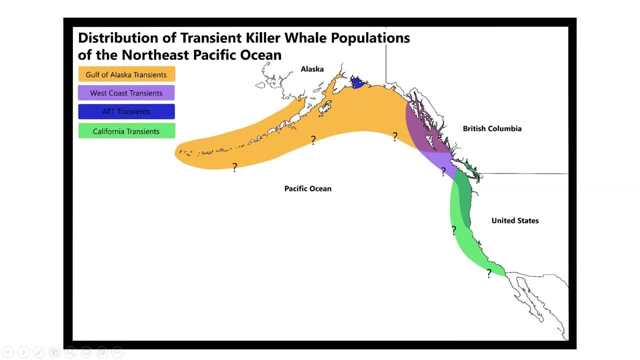 This population forms from southeast Alaska all the way down into British Columbia, Along the outer coast of Washington, Oregon and down to California And all the research we're looking into now. even though these are the best known, they're also the least known. we're starting to learn new things about their distribution. 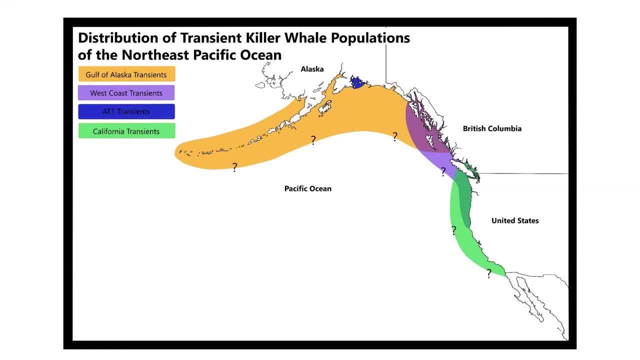 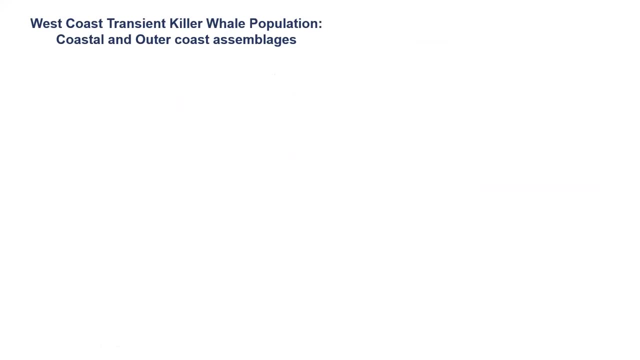 Potential subpopulations or or communities inside the West Coast transients that are, that are dependent, are independent and have their own habitats and characteristics, and that's a lot of the research I've been focusing on. And so just to kind of show you, here we have what we believe to be a coastal and outer coast assemblage or subpopulation. 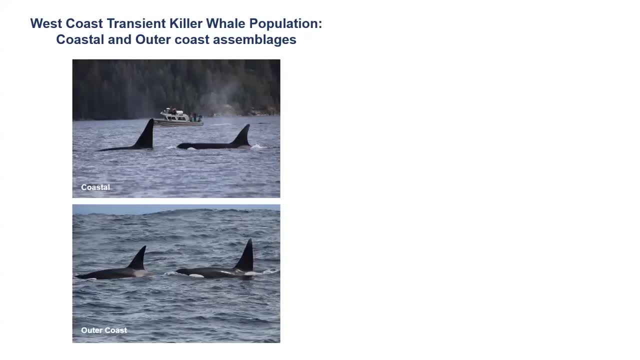 So a bunch of the research I've been conducting looks into this. We have a coastal group that spends most of its time near the coast in reef areas where there's reefs along the continental shelf margins, so areas where it's shallow water in inlets. 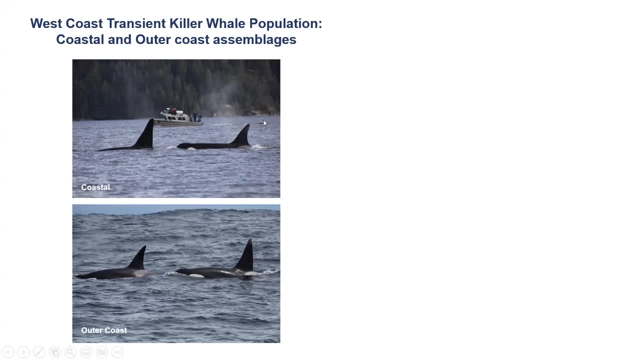 These are a lot of the transients we see along the coast of Oregon during the spring months that are that are predominantly eating harbor seal as well as sea lion. But we also have another group called, we believe, called- the outer coast, And this group is 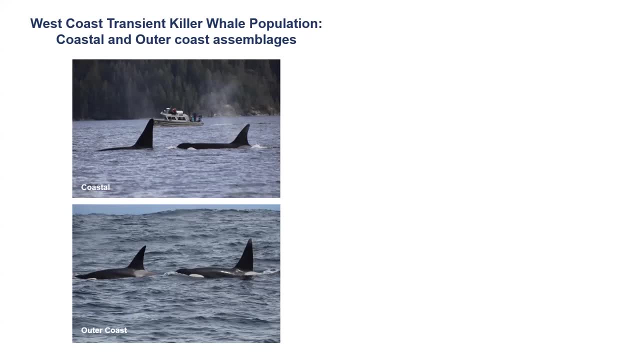 And this group we see most often near in the California waters or offshore of Oregon. A lot of our sightings have are from, and they are predominantly near, the continental shelf break, which is runs offshore just close to the open ocean, where the continental shelf dips off and and and goes out along the abyssal, the abyssal depths. 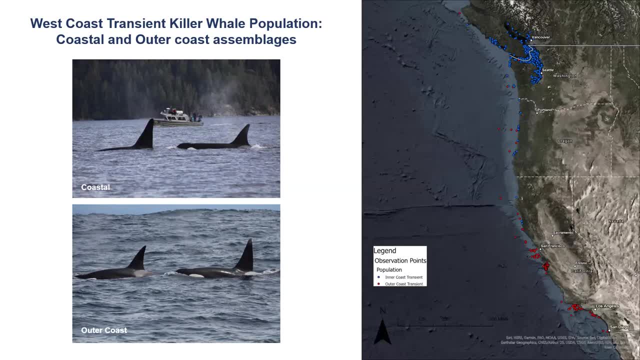 This is data that we plotted showing the distribution of sightings that we've collected for the West Coast population, and I just want to throw a thank you out to the Cape Perpetua Marine Reserve as well as the Oregon community, Because for a long time the Oregon coast here has been kind of a dead zone for sightings. 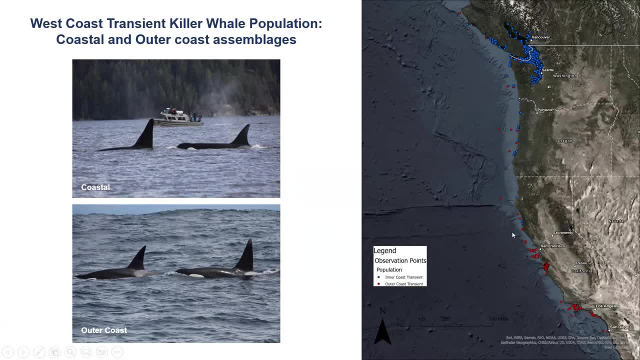 There hasn't been a lot of reports coming in And that became kind of an issue when we were trying to understand the overall distribution of how transient killer whales use the area, especially between these two kind of subpopulations. So for instance, off Vancouver Island, here we see a predominant. there's a lot of sighting networks, a lot of whale watching activity in the state of Oregon. 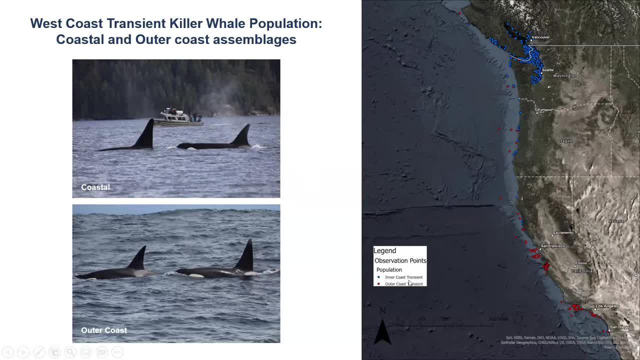 So, for instance, off Vancouver Island, here we see a predominant. there's a lot of sighting networks, a lot of whale watching activity in the state of Oregon We could see in the Blue Dots. here You can see those of these inter coasters of coastal transients that are found predominantly in here. 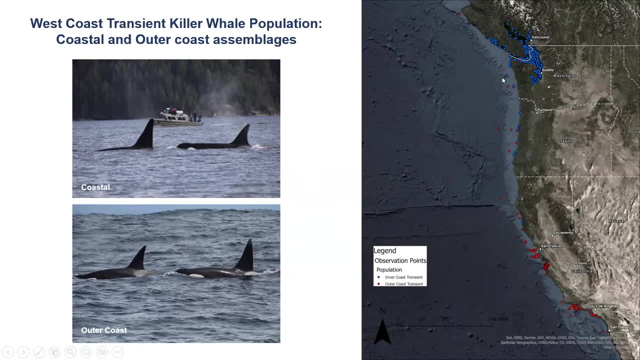 And then also we can see in the red. here the red dots are predominantly outer coast and you can see they're much more distributed closer to the shelf break And as the continental shelf- This is the shelf right here- you could see kind of running down the coast. 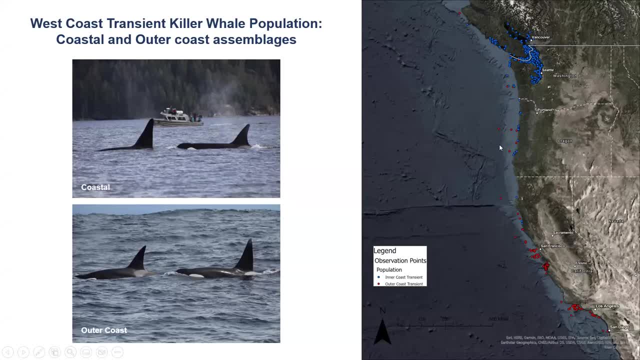 It's quite wide off of Vancouver Island in out coast Washington and Oregon. But as you head south you start to get a sort of narrow and bring into Monterey California, which is right. here that shelf break comes right into about five kilometers of shore at moss landing And this 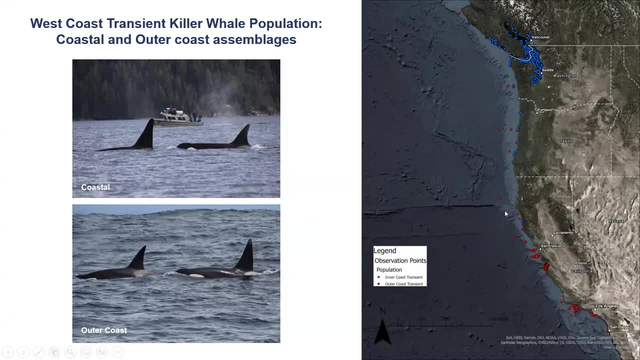 is where we see a lot of the outer coast. population is in these red dots in here, So they like deeper water further from shore. But both of these. what makes it even more complex is that, even though they're spatially distinct, we see more outer coast latitudinally south of you know, central. 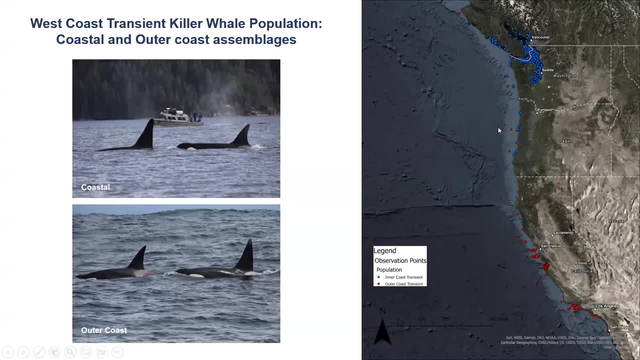 Oregon down to California. they do intermix occasionally And we do see kind of individuals from the inner coast and outer coast in each other's habitat. But we're still kind of learning about how these animals interact with each other. So kind of my interest for is 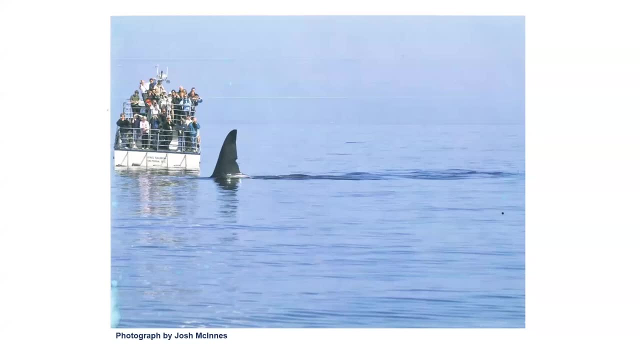 where my interest in killer whales, especially from the California and Oregon region, came from was that we knew so much about killer whales around the state- They were sea Vancouver Island- But we really didn't know a lot about what was happening in Oregon or California. And in 2009,, while I was on a trip to a field survey, I encountered a group of 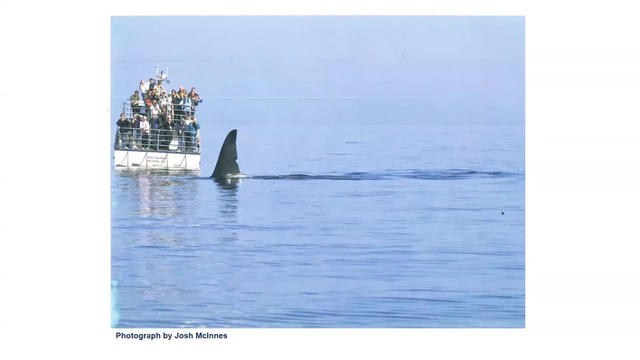 local inner coast transies that we knew quite well. They had recently killed a California sea lion and they were feeding on it. I got a report from a fisherman not too long ago that wasn't too far away And he said there was a big group of killer whales that were coming our way- about 25. 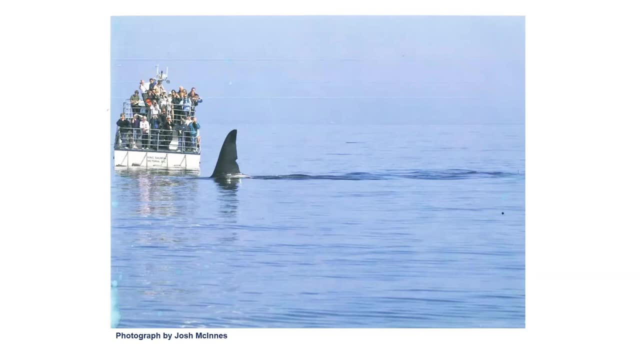 of them, And that was probably the first killer whale that we saw, And we were able to get a pretty exciting because we initially thought it potentially was the southern residents that were moving their way in through Juan de Fuca Strait, which is a body of water that separates Vancouver. 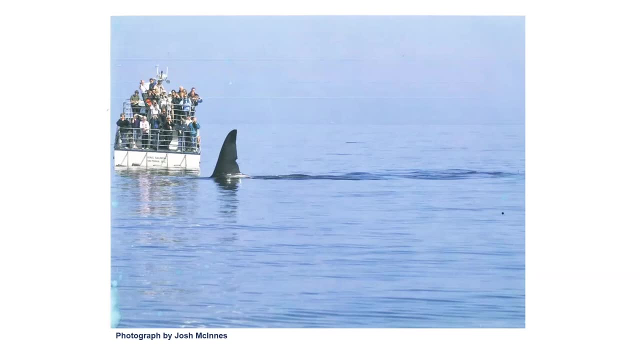 Island from the US Washington, And what we found was that when the group showed up, it was actually a large pod of transients, So we were shocked. It was actually over 40 of them. It was the largest group we had ever seen And we were photographing away and they were socializing And this 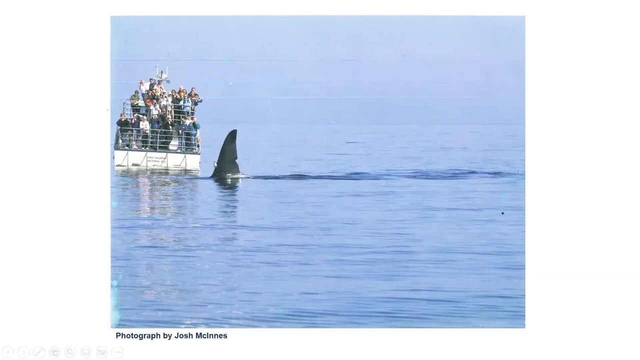 particular male that you can see in the photograph here. male killer whales get this characteristic large dorsal fin when they hit sexual maturity around 15 years of age, And this grows until when they're adults, about 20, 21 years of age. But this large male was not recognizable. 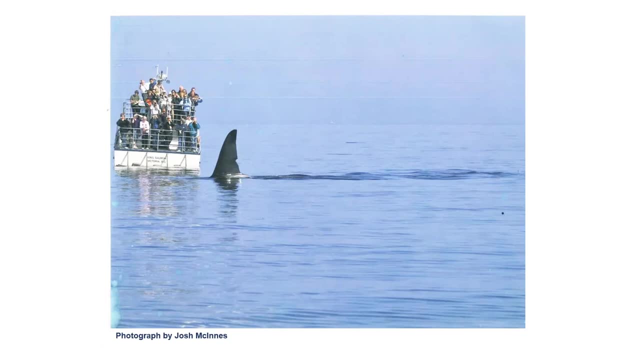 And as a research scientist, how we recognize killer whales are through photographs that are shared with our research team, And you can kind of see this notch here. This is particular to this individual. It's an injury that happened at some point And that notch stays with this animal. 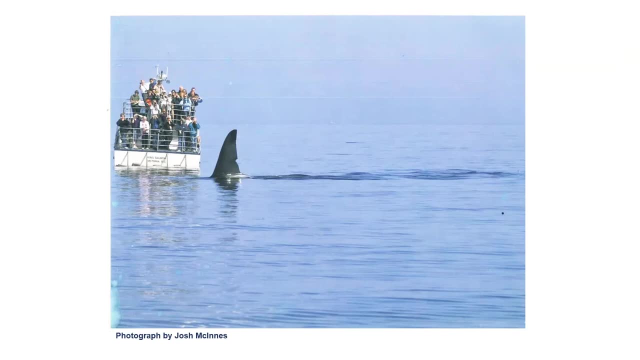 because it was unique. We had never seen them before, And so our research team took photographs of him and another female that we didn't know who, that we also didn't recognize, And it took us two months to find out that they were individuals that were most commonly seen off the Central. 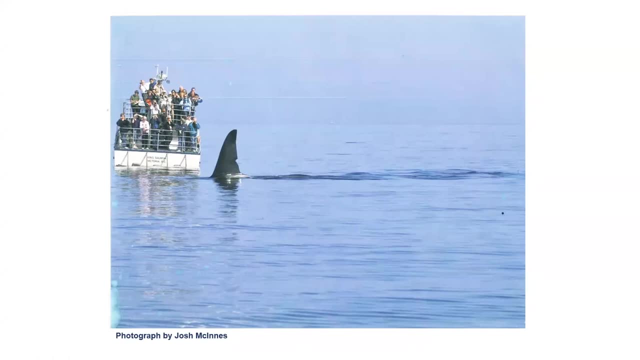 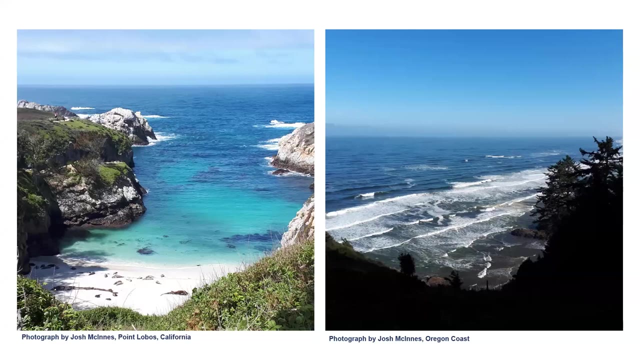 California Coast. So that kind of just really excited me And I wanted to figure out more about them. So we ended up talking with a nonprofit organization in Monterey called Marine Life Studies And I teamed up with them as the research coordinator and we decided to try to do a complete census of the killer whales in that region or a study of 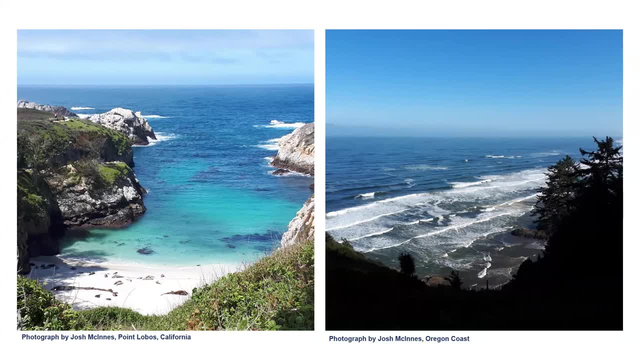 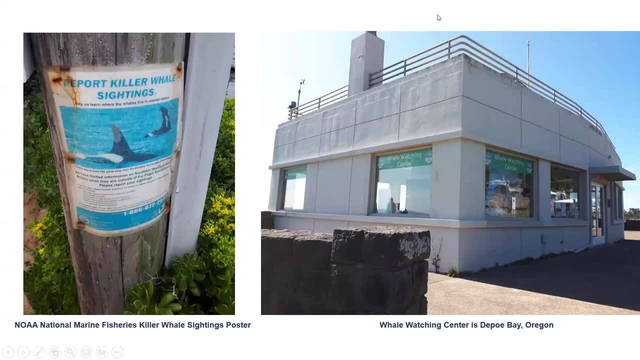 them. So I set off on an adventure. Two main study areas was the California coast and the Oregon coast, And we set up a pretty interesting study. We went down the coast. we visited locals in the Oregon area as well as in California. We talked to naturalists. You probably recognize this whale. 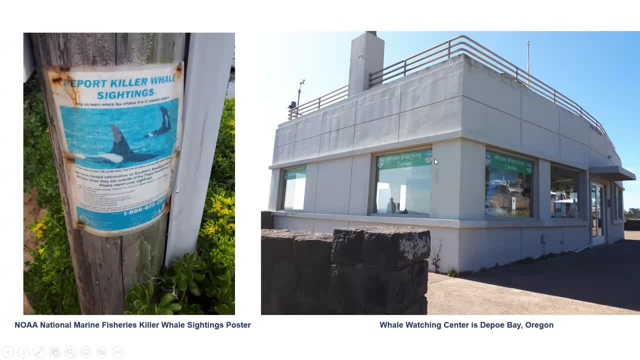 watching center here in Depot Bay. It's a great spot to watch gray whales as well as a lot of killer whales are sighted in the spring. We've got quite a few sightings in the Oregon areas in Depot Bay. But then also we talked to and collaborated with NOAA National Marine Fishery. 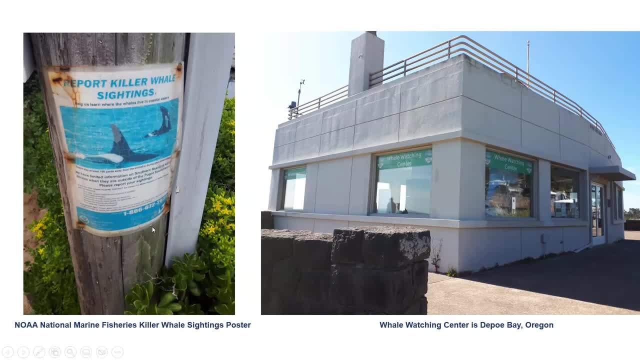 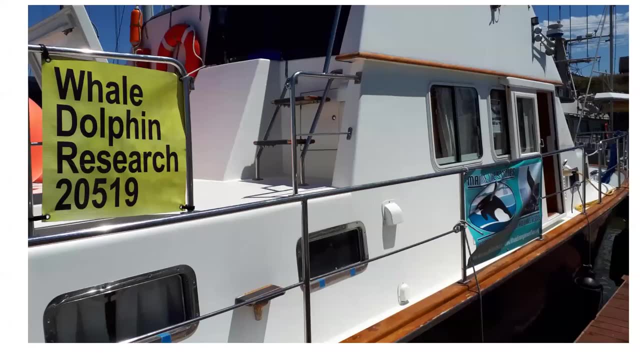 Service and coordinated sightings with them as well on killer whales being seen. So this was a bit of an adventure, a bit of a road trip down the coast. But then, finally, as we got to Monterey, California, where we based our studies, we teamed up with this research group called Marine Life. 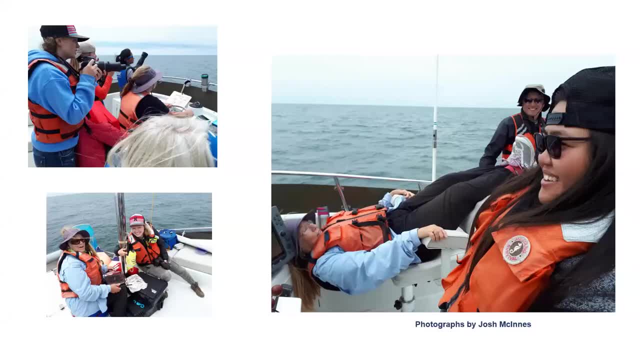 Studies And we had some pretty great time Between 2015 and 2020,. we conducted a very, very extensive study looking at the behavior of transient killer whales, which I'll share some information, but we have naturalists that were on. 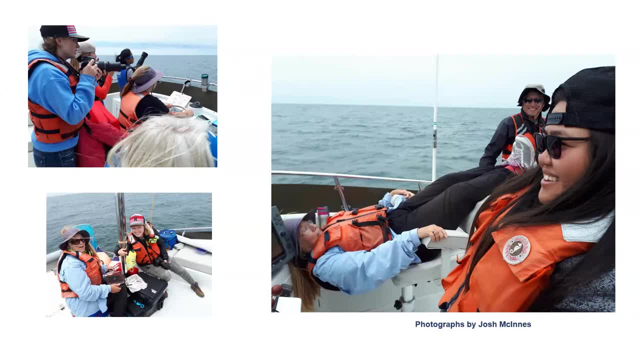 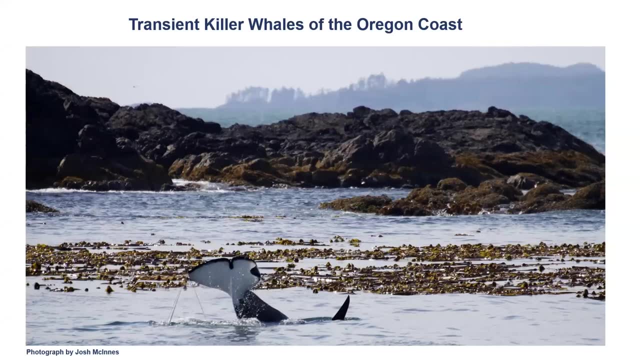 board biologists and that we worked together to collect this data over this long period of time. So what did we find? So first I want to want to talk a little bit about the Oregon coast and and killer whales, And it's really exciting kind of what we're learning. 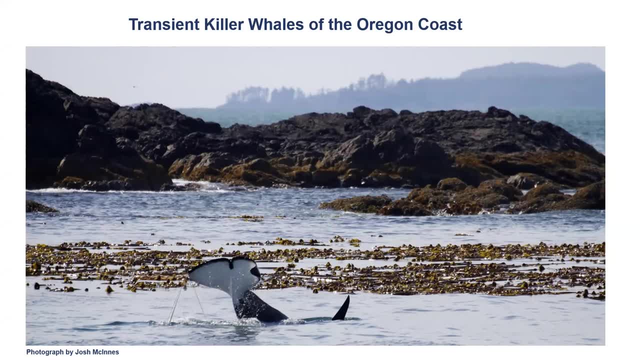 And, as I mentioned earlier, it was a bit of a dead zone when it came to sightings. A lot of people, a lot of scientists, are focused on gray whales off Oregon because they're just so much more prevalent and accessible. There's quite a few that are residents to the area, But killer whales are. 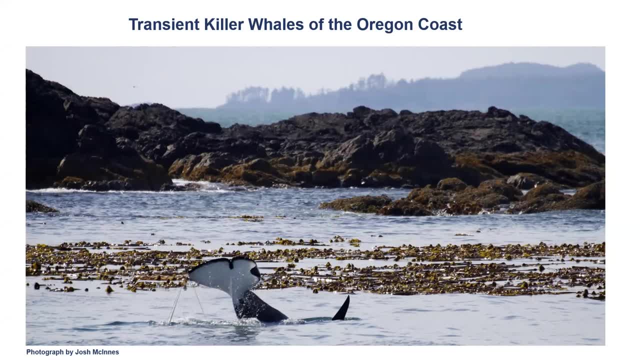 kind of harder to find, And a couple of reasons for that, One being the weather off Oregon can be quite rough. It can be quite difficult to find animals, especially with the big open ocean. Their killer whales are a lot smaller- smaller than gray whales- And they 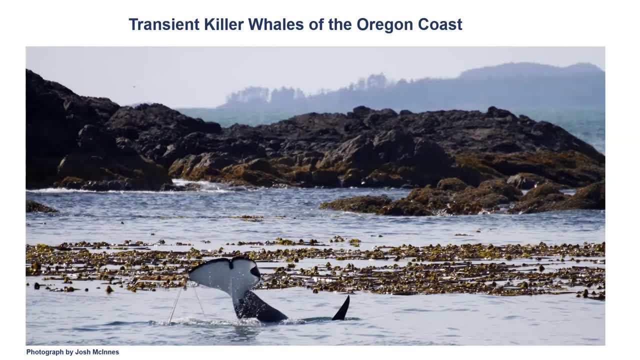 typically move through the area quite quickly and they don't linger for too long. The other reason, though, is that there hasn't been really any dedicated research on killer whales off Oregon, And a lot of local Oregon people often collect information, but it might stay or sightings. 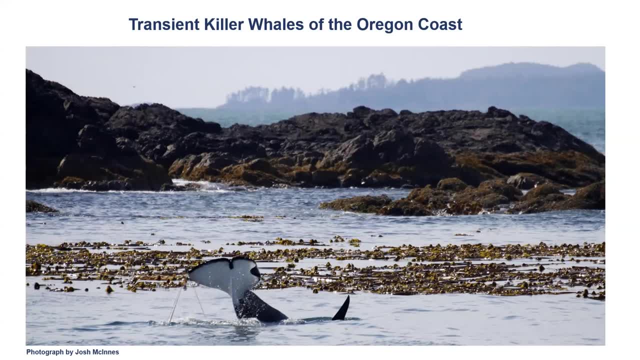 but it might stay in their private database because there's nowhere really to share that information. So in 2021, we formed a social media citizen science initiative to collect sightings of killer whales And we call it the Oregon Coast Killer Whale Sightings. 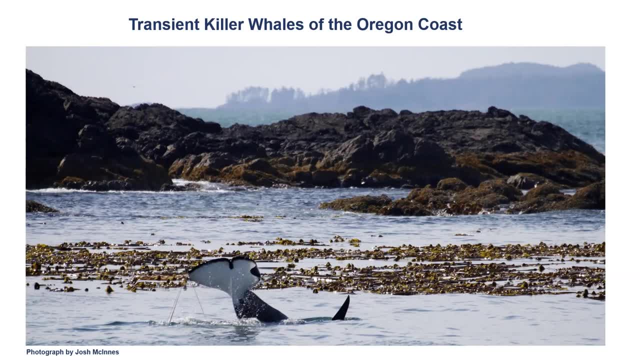 Group, which is part of our Oceanic Ecology Group research project, And it's been very successful. We've been able to collect hundreds of sightings, not just recent sightings of killer whales, but also historical photographs that people like fishermen, naturalists, park rangers have. 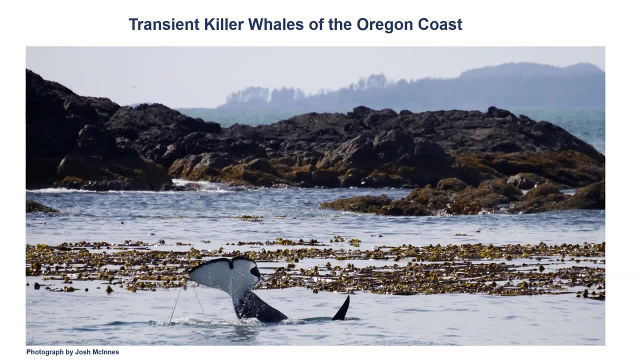 encountered have sent in And we've been able to- really we've been really able to- open up the area of Oregon and connect it to the rest of the region of study that we've been looking at the distribution of that West Coast population. So this outer coast is a lot more difficult to survey. 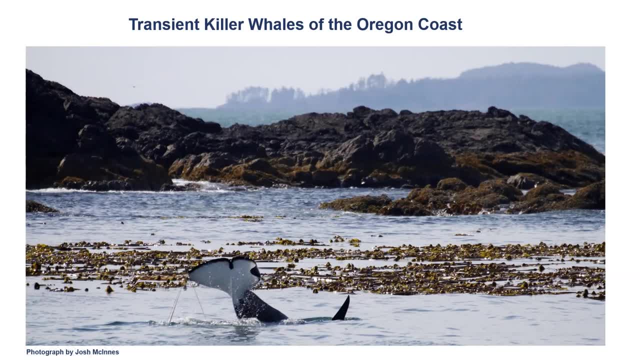 but we're we're learning more about it And I can tell you right now the group is up to 7.8 thousand Oregon locals, which is the group is is strictly for people that are in Oregon, that have the opportunities to see whales on a daily basis, And we're learning so much more. 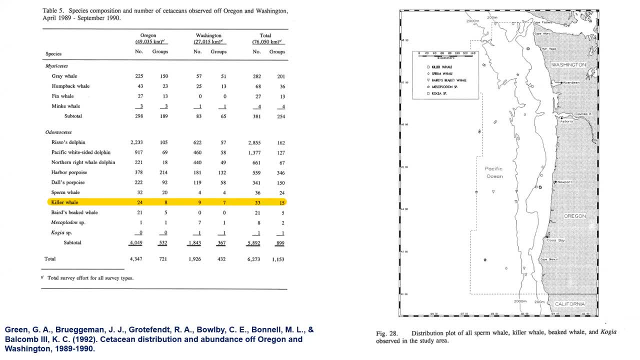 But the first historical studies of killer whales along the outer coast really kind of spiked my attention when I looked at the literature. This was a paper published in 1990 by Green et al And it was a report that looked at the abundances of marine life in 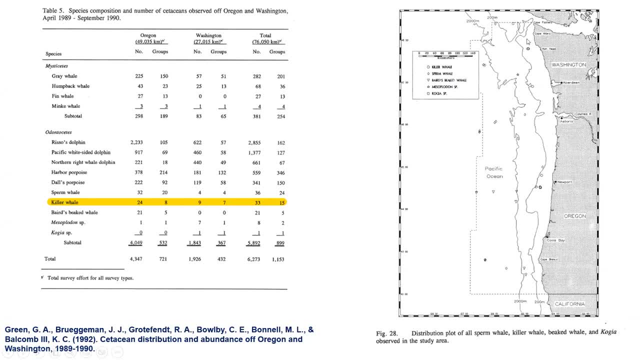 particular gray whales, marine mammals and particularly gray whales along the outer coast of Washington and Oregon. So it was focused on gray whales but it had many other species And this was based off aerial surveys through airplanes that collected sightings And what you can see. 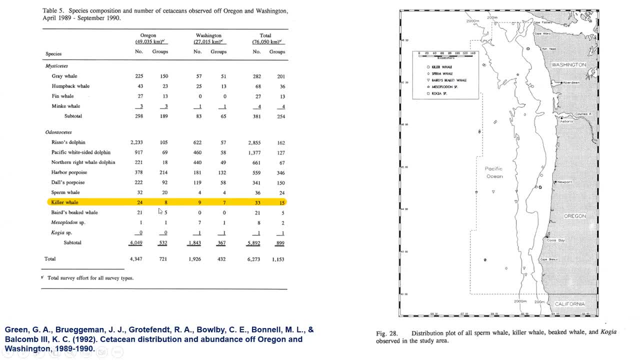 here is killer whales 24,. you can see there was quite a few animals but none were known, And in this report they they was collaborated by scientists that were studying killer whales in the inland sea. Most of the individual killer whales that were being sighted were not able to be matched through the 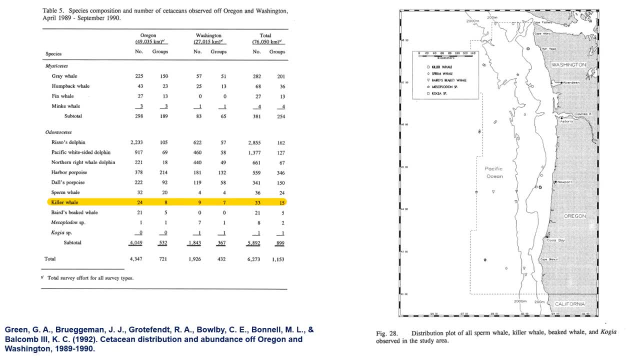 photo ID process to individuals that were known. So these were unknown animals So, but unfortunately that information never was really known about if they were offshore. 00,12,13,14,13,15,16,17,18,19,20,21,22,23,25,26,27,28,29,30,31,32,34,35,36,38,39,40,34,39,41,42,44,45,47,48,48,48,49,52,45,47,49,49,50,51,50,52,50,50,50,50,55,50,50,53,56,56,57,58,59,59,55,58,59,59,59,59,59,59,59,59,59,59,59,59,20,50,56,58,59,59,20,52,25,56,00,00,00,00,00,00,00,00,00,00,00,00,00,00,00,00,00,00,00,それ que. 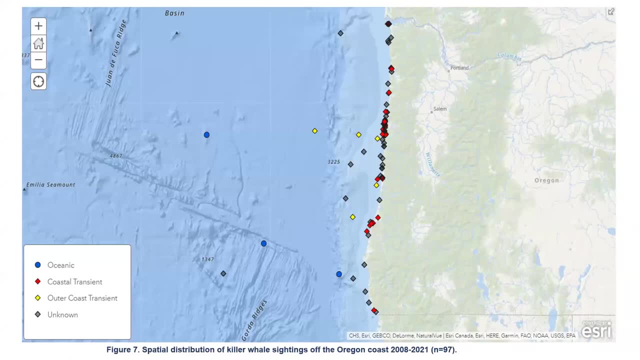 So what have we found? So here's a spatial map looking at the number of sightings of killer whales along the Oregon coast, And that's 97 sightings from 2008 to 2021. And that's actually quite a bit. in particular, when we're looking at the most recent, in 2021- actually 2022- we've had an up, an increase of around 50 animals, 50 sightings, which is even more exciting. 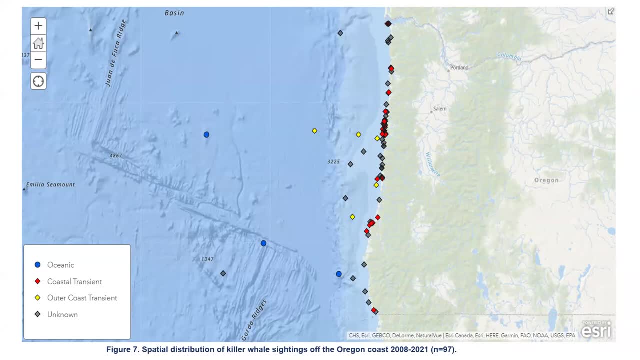 I think that's a lot of the fact that we're our effort is increased with with the ability for the sighting groups to form, As you can see here, though they're separated on different kinds of killer, different populations of killer. So we have this unknown here where people have sent a, sent in a report but weren't able to get photographs. 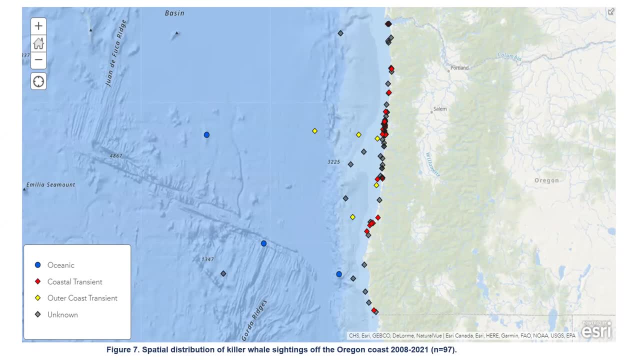 And unfortunately we weren't able to positively identify. we just know that there was killer- was cited that information- still important as it enables us to look at presence data. that we know that killer whales were in The area, which is important. it shows some sort of habitat use, but we also have animals that we were able to identify, which is the most important form of data. 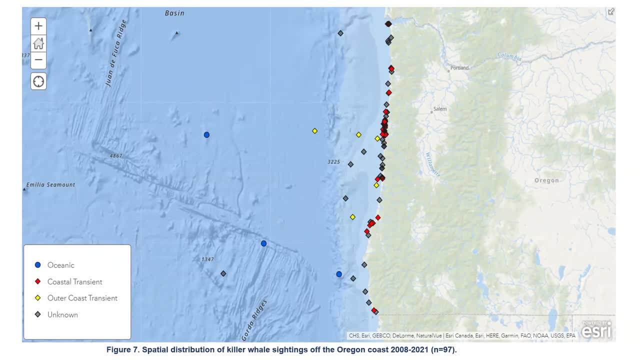 Which is photographs that we've been identified on the dorsal fin and saddle patch, which is unique to each animal. So the coastal group here in red are those inner coaster coastal transients and you can see they're really focused along the coast here. they go right into areas like the canals and along the jetties off of Newport and Florence and we get a lot of. 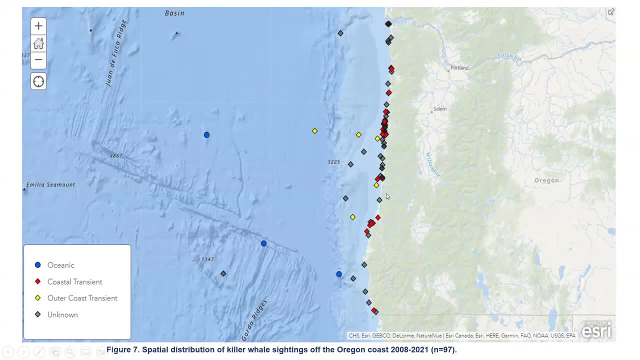 sightings where they're searching for seals, they'll go way up and even up into coos Bay, up into the river there. And then we have the outer coast, which I mentioned, which are yellow you can kind of see. they're more spatial. The distributors not as many, but that could be just effort related, where we don't have a lot of people that are actually out here along the shelf searching, so we are likely not getting a lot of sightings that are out here. 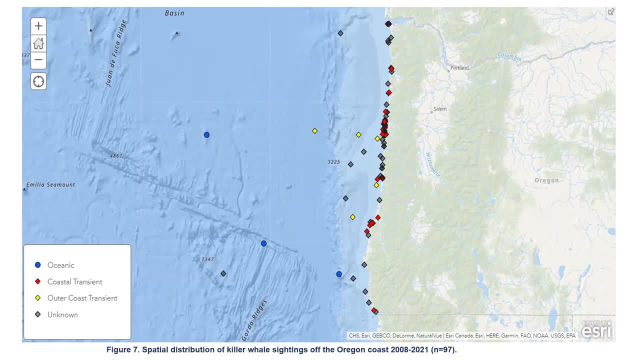 So the more important that we collaborate with the fishing community and pelagic birders that might be out there doing surveys. And then we have this blue dot here and i'll explain a little bit about that in a further a couple of further slides down. but this is an important we call these killer was ever seen on your oceanics. they're mostly seen seaworld of this show. the continental shelf break here further offshore, and i'll talk a little bit about those in a few slides. 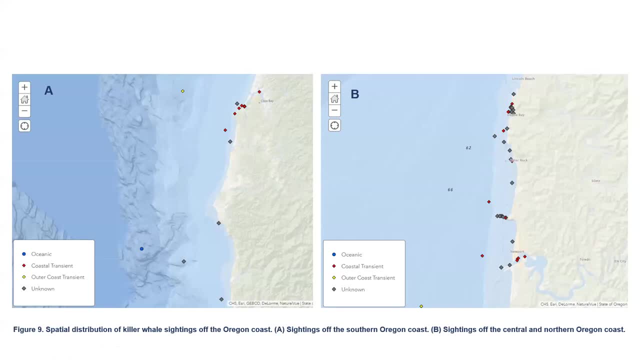 So this is kind of the coast broken up into two halves, on more northern Oregon and in central Oregon here and then the southern Oregon coast here With how those same Sightings are kind of distributed. but you can tell that there's there's a lot of effort in certain areas, like more settings occur in coos Bay or depot Bay. 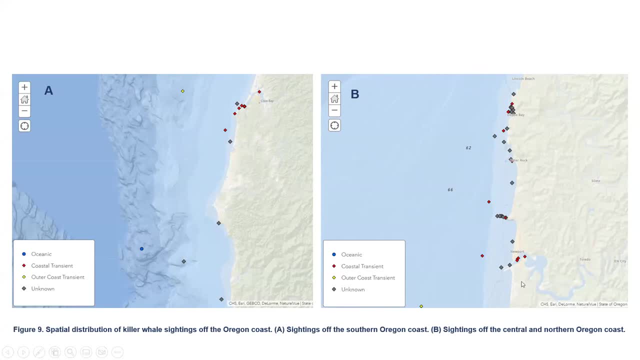 You know otter rock area down in newport and this is majority or the majority of the population live on the Oregon coast or in these areas And we're a lot of the whale watching effort. is but likely that we're missing some of the settings that are occurring along these other stretches of the coast? 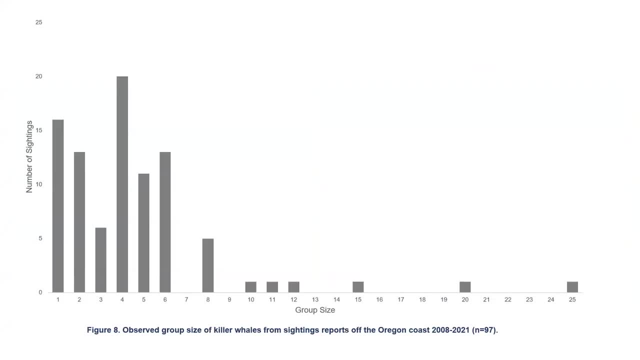 But the encounters with killer whales have involved group sizes And these are mostly just With the transient killer whales we've been seeing groups of about four to five individuals on average. then that's typical for transient killer groups that we see, But we also see down here even larger groups of 25, so this is group size along the X axis and then on the y axis number of sightings and you can kind of see sometimes we do get large groups that do form. 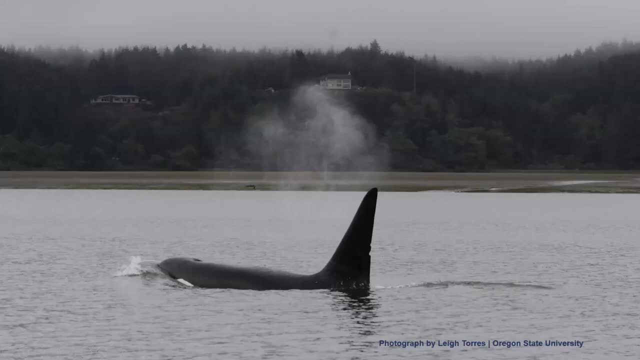 Of killer whales. so there's a photograph from our colleague Lee taurus at Oregon State University. This is T 49. See, I mentioned him earlier. he's kind of a local favorite for quite a few people that got to know him. you can kind of see his two notches here that are characteristic for him he's. this was just outside newport and he was moving his way in through to the jetty looking for seals. but how we identify killer was I'll explain in a few slides as well. but this is a. this is his number and his name. 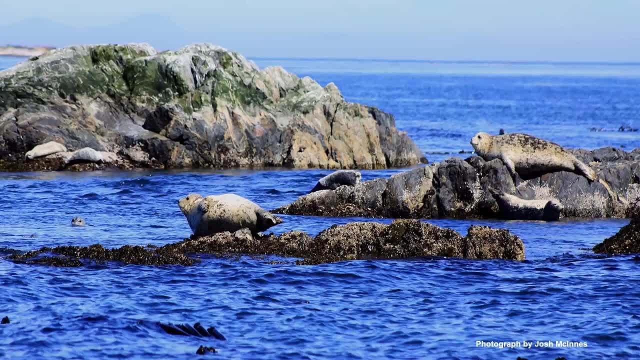 So why are we seeing so many killer whales? this is a question that i've been getting asked by a lot of people that are following Our research along the coast. why are we seeing so much? is it increasing, or people you know, particularly the last year? people have been asking: 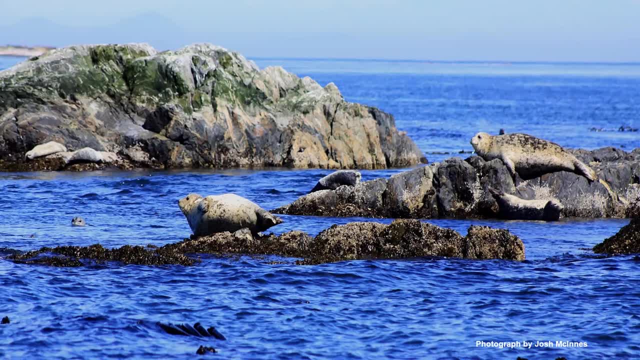 Oh man, is it josh? have we seen more killer was? is there? is there a reason for it? there's a couple of I have possible hypotheses that we're looking into, one of them being, as I already mentioned, it could be effort related. more people are looking, more people reporting to have a sighting network to report these settings to. And that could be one reason, or the other reason could be that we're seeing a shift in the prey population and, as mentioned, the coastal transient group is increased over the years. but they are mammal hunters and their main prayer what we call harbor seals. 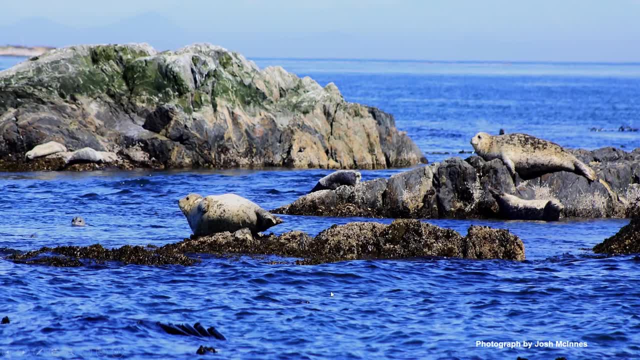 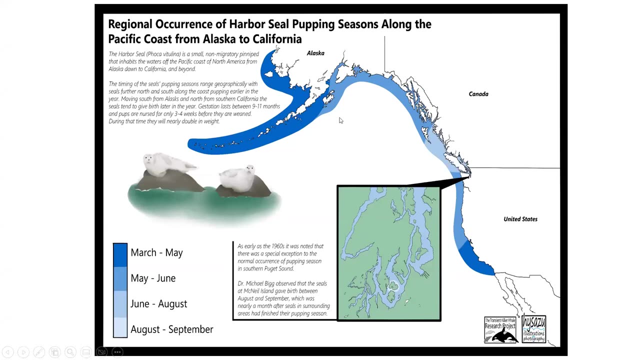 And they also for john sea lions and porpoise. but harbor seal is really the species that has driven the population growth over the last few decades, especially in the waters around southern Vancouver island. But harbor seals had this climb along the coast. so the blue shades on this map we created show the differences in. 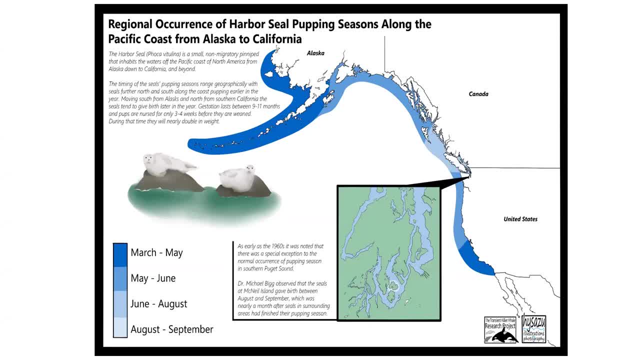 When the popping season occurs- so early studies in the 1990s really highlighted transient killer will occurrence, or when they show up That it was related to the harbor seal popping season in the waters of southern Vancouver island, the US San Juan islands, And that peak in the season was around between August and September and transient killer will increase their time in there. 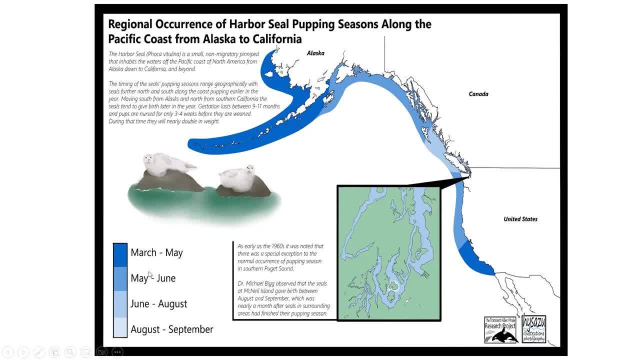 But what we're learning about the Oregon coast is that most of our sightings of transient killer whales have been through basically March through May, and that is also around the same time that we're starting to see the pups being born off the Oregon coast. 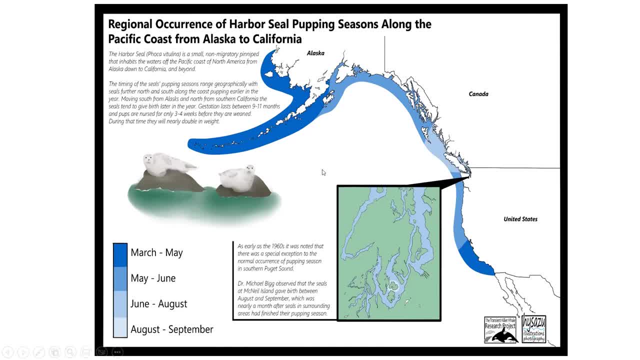 So, and with the increase in the sightings that we've been getting and people learning about how to photograph killer whales, so we get the ideas of animals- we're learning that some of the groups that we're seeing off Oregon kind of shift their distribution along the coast up into the areas of southern Vancouver island, timing this difference in their movements between Oregon and British Columbia. 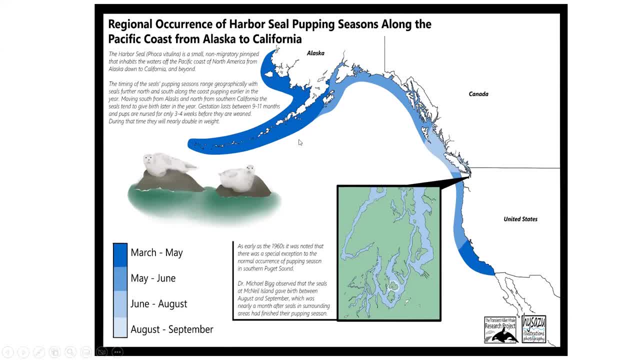 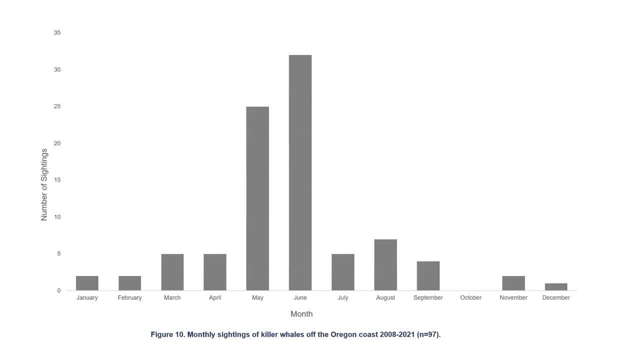 So there could be A client also in. the killer was following their harbor seal popping season. but we're kind of still in the infancy is this research, trying to learn a little bit more about it. But as you can see here in this graph on the X axis here's the month and then the y axis is the number of sightings and you can see in May and June is kind of the height of when we start to see. 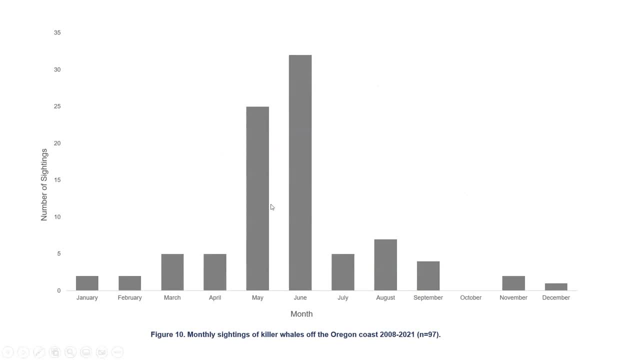 pups being born are sorry killer was being cited and that's as I go back. you can kind of see that's during this period of time or harbor seals are being born off the Oregon coast, So we're kind of working on trying to correlate. 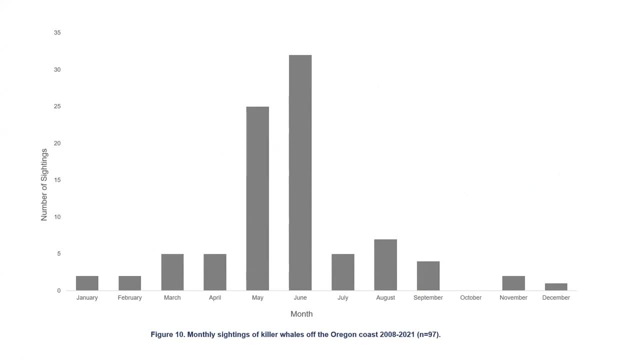 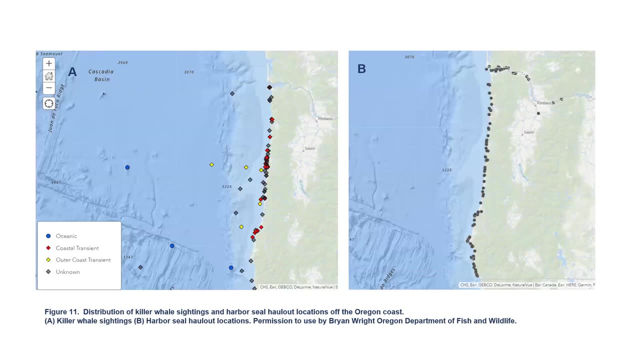 This to understand if there is some sort of relationship between harbor seals and killer whales, similar to what has been studied with the population on off southern Vancouver island. To do this, though, we're kind of been teaming up with them to Oregon Department of Fish and Wildlife, who are responsible for managing and assessing the harbor seal population, as well as other pinniped species. as you can see, here is the same map on the left here with 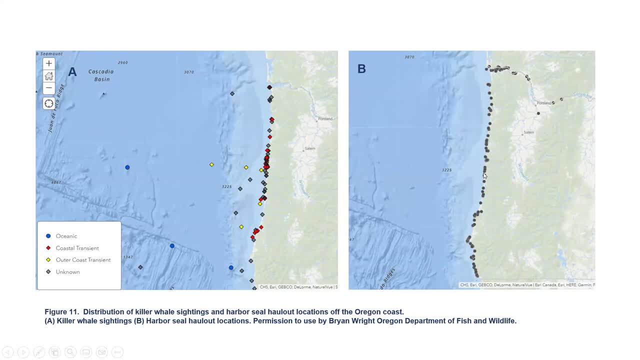 The killer was saying: but on the right here is The locations of where harbor seal hollowed. so hollowed is where is a rocky substrate similar to like a reef. it could be a cobble beach. it could be On a log boom. it's an area where seals will come out to rest, give birth or molt, which is getting rid of their fur. 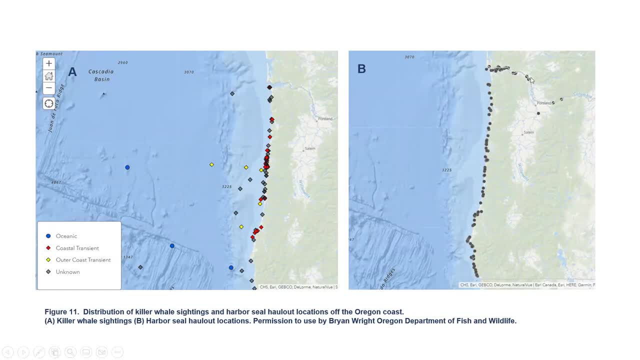 And you can see it in a concentration sometimes between 10 to over 100 animals. but you can see harbor seals, areas where harbor seal seem to to use their spend their time, which kind of overlaps here with a lot of where we see the killer well sites, especially for the coastal transients. 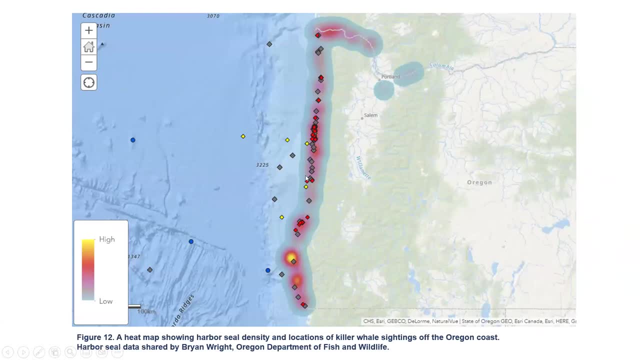 And as we kind of look at this, this Is a heat map, looking at these sightings again, but also looking at the heat or heated areas are where we see the greatest abundance of harbor seals, As this the word the heat is, so there's high abundance is the lighter colors were, the cooler colors are. 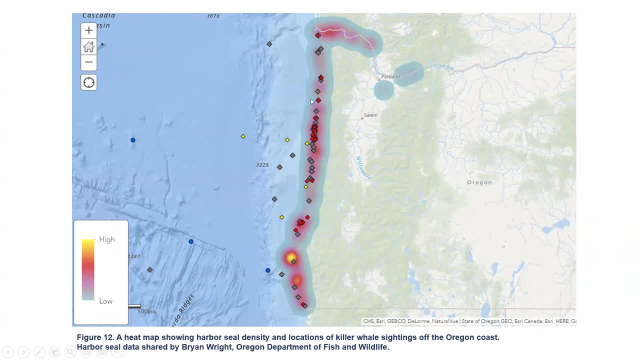 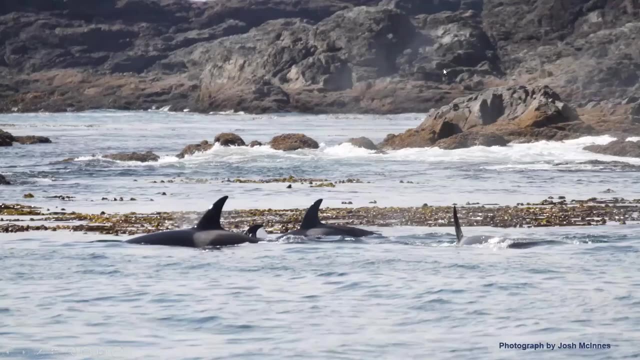 Less abundance. but you can kind of see here, especially in areas where it's kind of medium to high, we see a lot of killer whale occurrence and and most of these great unknowns are likely transients. we know So foraging behavior for transients, especially the inner coasts. they spend a lot of time in quite shallow. 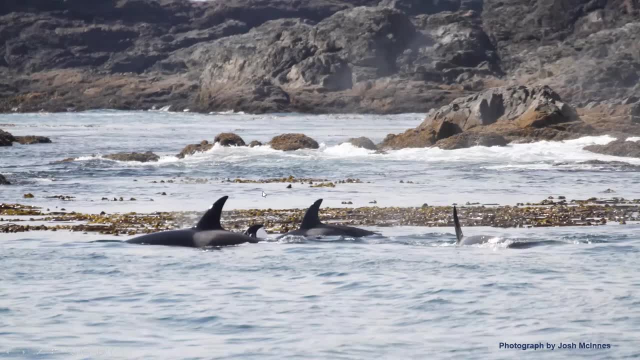 Water. so if you're looking out over the ocean, the open ocean off the Oregon coast, and you see these little islets or these little small ocean islands, there's chances you may find killer whales searching here. this is an area where harbor seals will haul out, as mentioned on these little reefs are on these rocks. 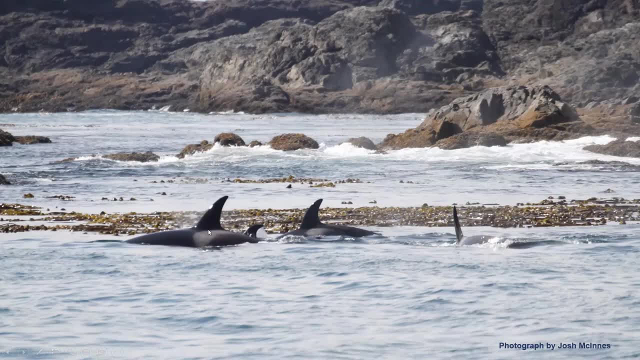 And killer whales will come right into the kelp bed, searching sometimes in the water that's only five to six feet deep. it's it's not surprising that we see them. so this is kind of a family of transients that are coordinating their hunting, looking for seals in this area. 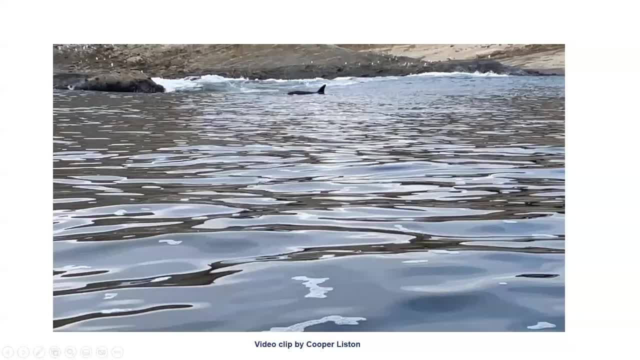 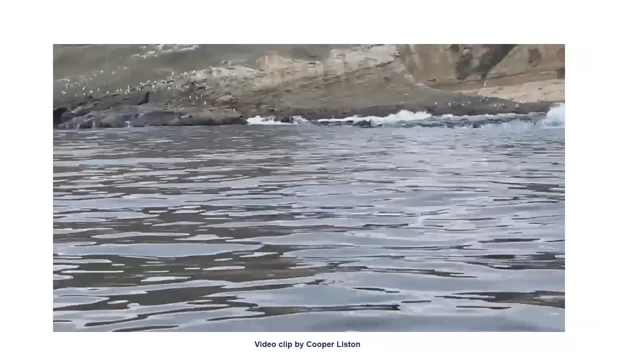 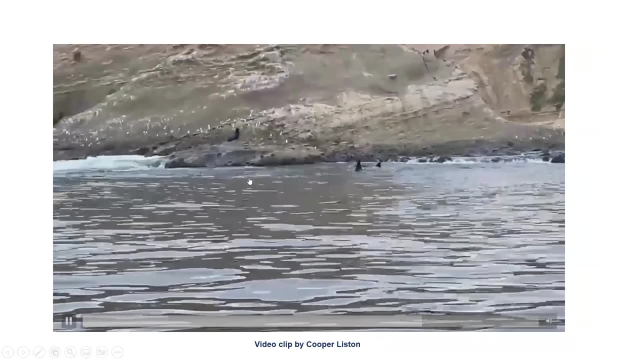 And here's A small video clip that was shared by a fisherman off of- I think was off of- Coos Bay that encountered some transients hunting And you can kind of see a sea lion up here trying to get out of the water, but you can see the real close following contours of the land hoping that they'll find a seal. that's, that's in there. 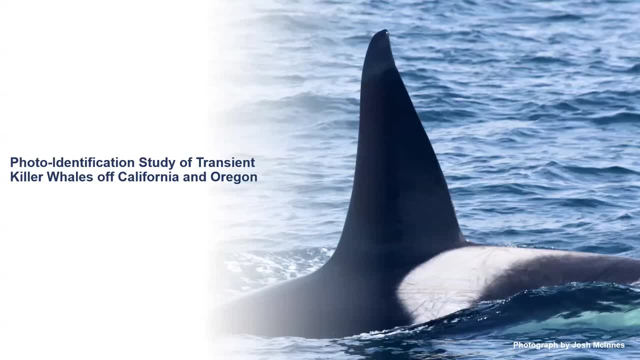 So the next part of this talk I want to quickly go over is the photo identification process. So the one of the big steps was trying to understand, as mentioned, what Is the killer whale population- like the outer coast killer whales that are less known compared to the inner coast- what was their population really looking like? and 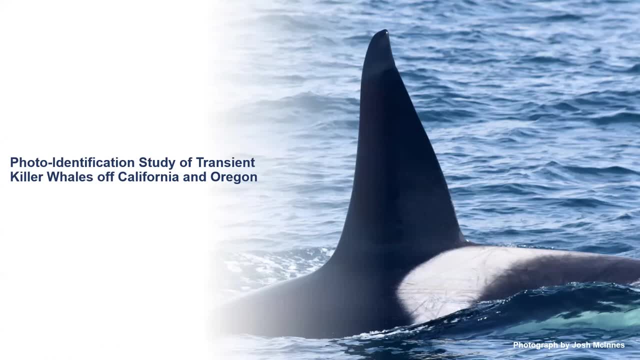 And what was the popular, what is the population like off Oregon and California? so how we do that is we take a photograph or we look at photographs sent in from the public or from the Community. and this is a dorsal fin here and you can see the saddle patch, these scars. 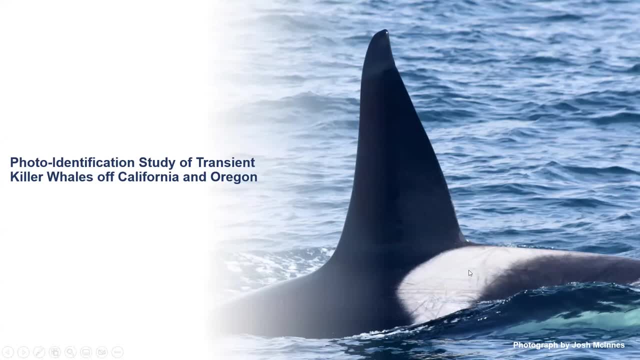 These congenital features are unique to every killer whale in the population and they don't change. And even the shape of the fin- you can kind of see here this mail, this thing kind of goes up in here- this animal, this, these features stay with the animal for throughout its life. so we, we census or catalog every single whale. 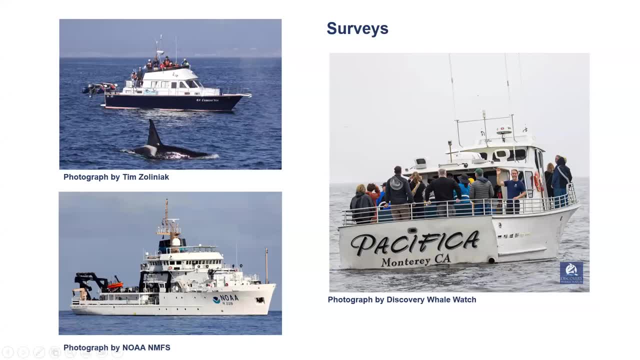 And we do this through a few different methods: one from the general public, but from some of our own work where we did opportunistic surveys off the California coast and Monterey, But also from a collaboration with the National Oceanic and Atmospheric Administration through ship based surveys offshore to really access some of those areas where we can't get a lot of information. 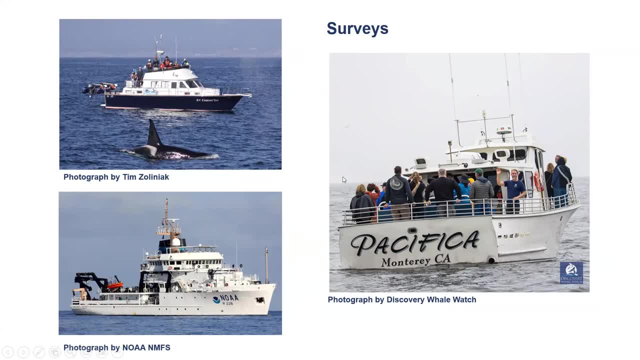 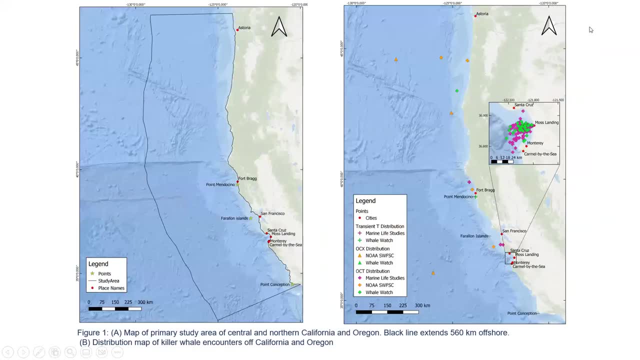 But also through whale watchers, that naturalist to take photographs during expeditions. we've been really we've been, we've been able to really collect and consolidate quite a bit of data And our study area was quite large. you can see here on the left map it extended from Point Conception, California, out to about 560 kilometers offshore, well west of the continental shelf break, all the way up to Astoria, Oregon. 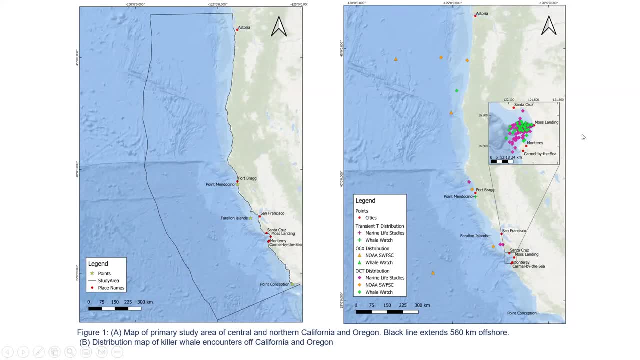 And then over here you can see, is the different sightings. so this is Monterey, which Is one of our main centers of operation, but we're proud to say now we're kind of focusing a lot of our attention in Newport as well and and the future studies will be in Newport, Oregon, as well as Monterey. 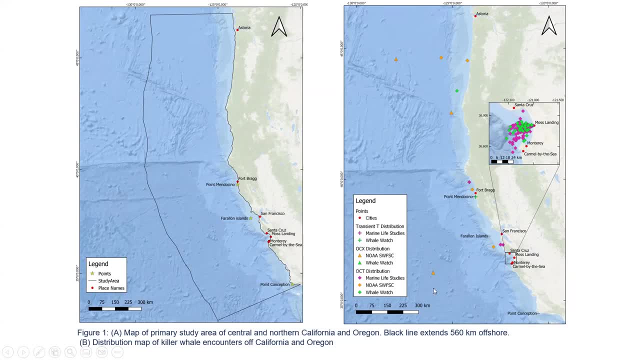 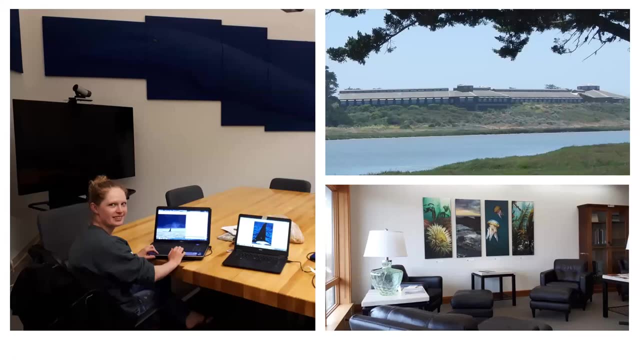 And you can kind of see here the differences in in The differences in effort, in types of organizations that collected these sightings. But it's not fun and games going out there all the time and taking photographs and watching whales. most of our actual work involves sitting behind a computer. 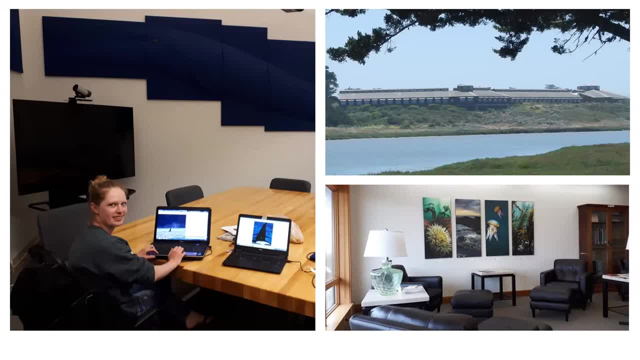 And for the photo idea effort we worked on from 2006 to 2018. This is what our photo ID study was focused on. that time period, we had to analyze hundreds of thousands of over 100,000 photograph Photographs, as well as spend countless hours looking through emails of people sending in images and moss landing. marine laboratories here in Monterey was very kind enough to lend us and donate their time at their library, as well as their equipment for us to sit and actually look through. 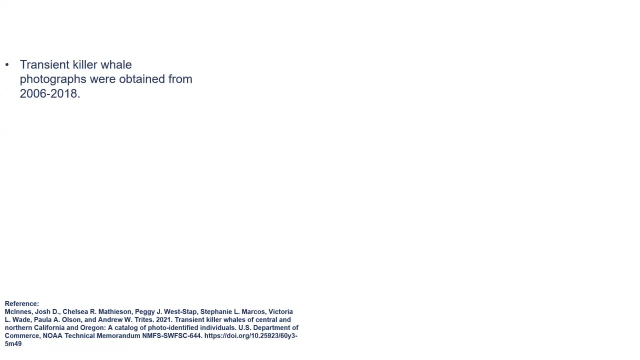 This large database. So what do we find? so transient killers were were photographed in. photographs were obtained from 2006 to 2018. we had over 146 encounters or opportunities to collect information on killer whales. we looked at 113,127 photographs and analyze those, and then we found a total of 150 individuals in the outer coast transient population that were distinct from 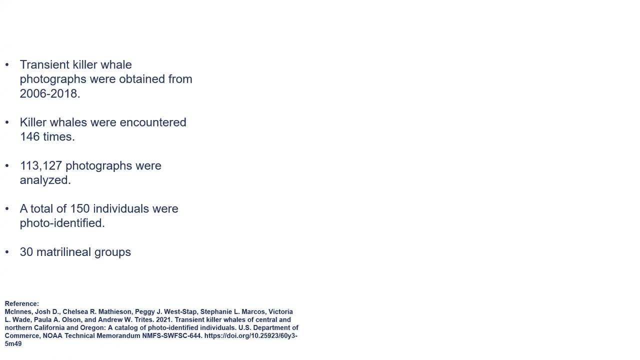 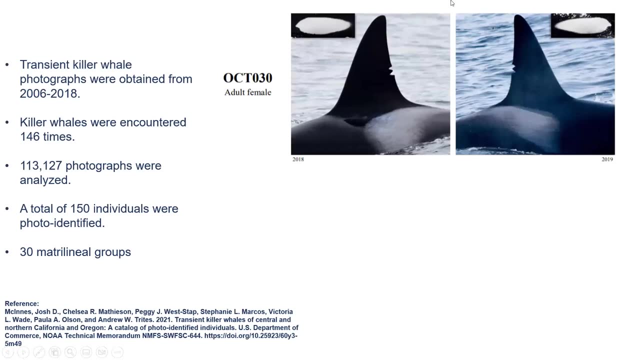 any of the individuals typically found in coastal waters, And this in company: 30 matrilineal groups or families comprising a mother in her offspring. So you can see here, this is how we identified an animal. we, this is a female we know as Emma, or OCT 30.. 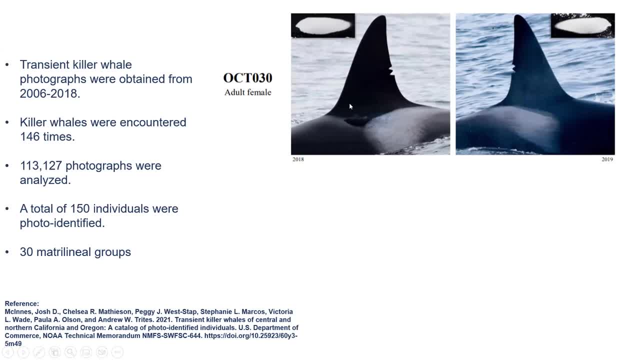 She has these two unique marks right here. she's not quite well known off the California coast, but it's also been cited off Oregon. We can identify her based on just this alone, but we can also identify her off her eye patch. this is the post ocular patch. 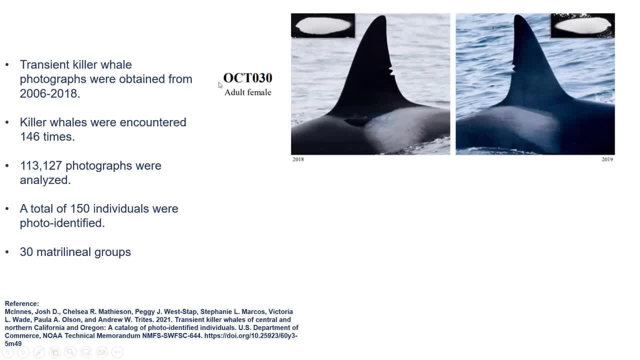 The top, her. I would sit just behind here. but we give each animal and identifier. so OCT literally means outer coast transient, and then the number 30 is her, Her number. So for instance, here we go: OCT 30 is the, is the female here the leader of the matriline, her family? if she has an offspring, her first offspring would be OCT 30, B or A, and her second offspring would be OCT 30, B and C, and so on. 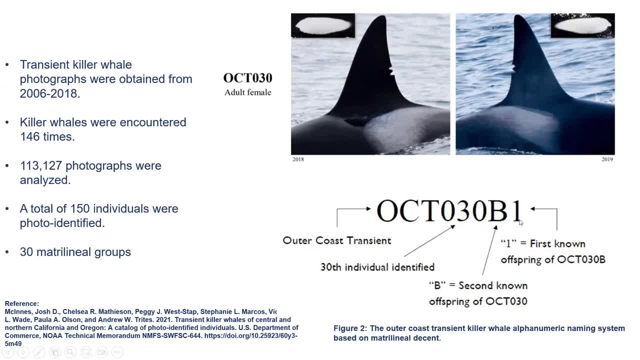 Now, if her offspring had an offspring, it would be B1, so be the first offspring, so her grand granddaughter or grandson would be given the B1 and B2, B3, etc. and we can do this for every single family as we get to know them over multiple encounters. 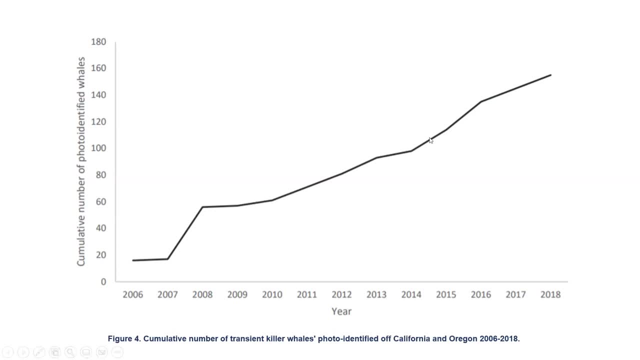 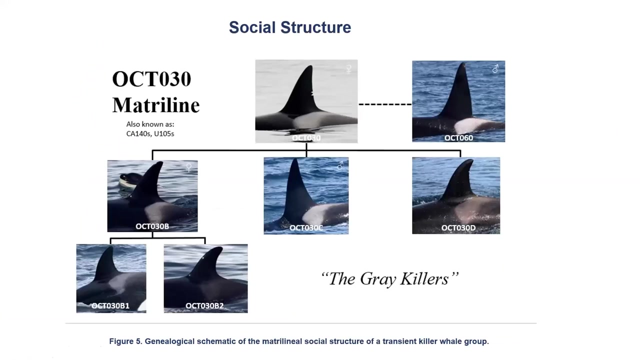 So what did we find? we found that throughout our study, there was an increase in the number of individuals identified, And this is both through births of new calves as well as new individuals being identified from Previous that have not been previously recorded in our study or published information. and this is what a family looks like, so you can see. here's the mother. this is OCT 30.. 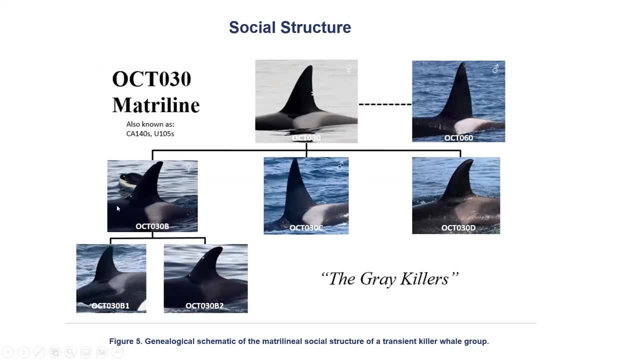 And then her first or second offspring. her first offspring died, so the second offspring would be: B, Her two grandchildren B1 and B2, her first son, OCT 30. C- her presumed brother- you can see the dashed line here means presumed. We believe this is her brother- 60. and then her fourth offspring, D. 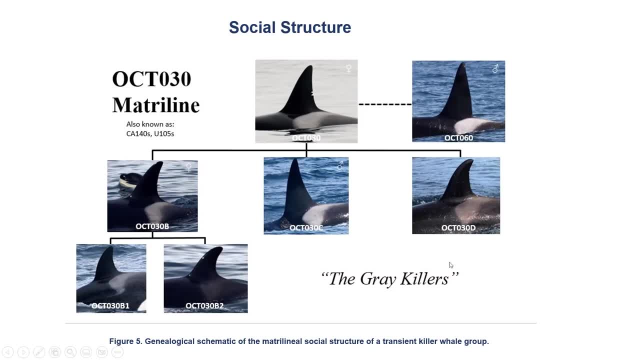 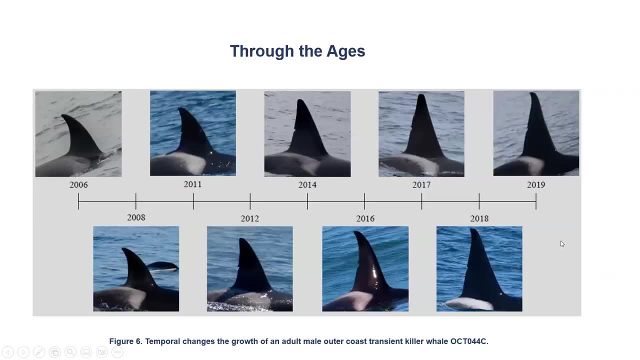 She actually has one more and we know this group is the great killers. they're very common. they're they're very commonly seen or encountered hunting gray well calves in Monterey, California. This is over the time period of this one individual we knew. OCT 44 C. 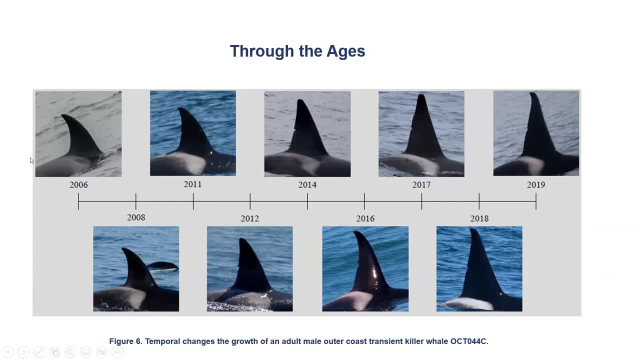 So it's so important when we get these photographs from the public that we can identify these whales because we can kind of track their life. In particular, this animal here was quite young in 2006 when we first photographed it And over time you can see it acquired a notch here. 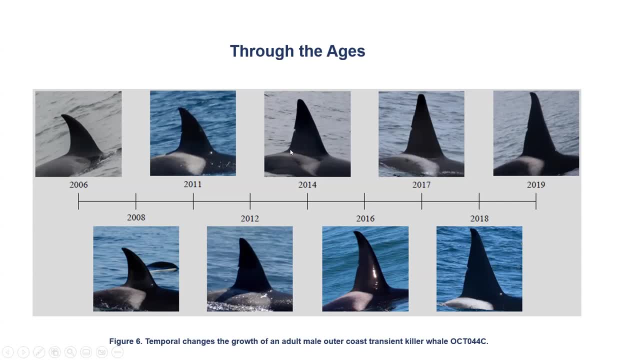 And then down here that is kind of starting to grow bigger. and then, 2014, it started to sprout this dorsal fin and then over time you can kind of see to being a full adult male. here that is sprouted in a sexually mature and physically mature. 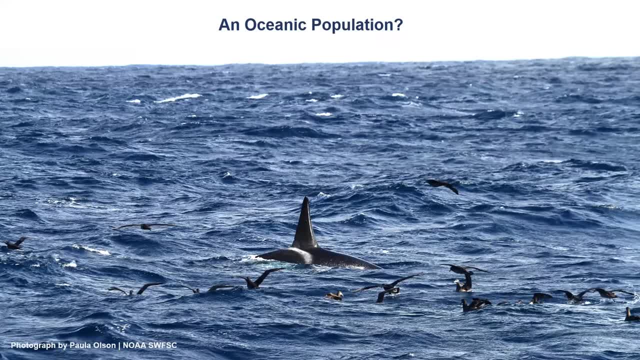 So I mentioned the oceanic population. so this is what's really interesting is that through the study, we found killer whales that were unique in the fact that they were not able- we weren't able- to match them through association to other known transient killer whales. 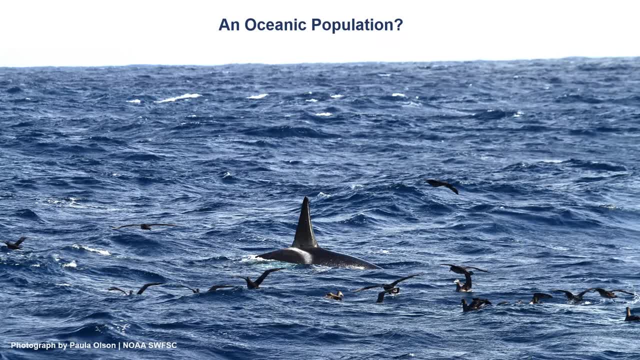 Or they were never seen in coastal waters So we really don't know what they are. But most of these encounters happen seaward of the continental shelf, far offshore up to three, sometimes up to 370 kilometers. You can see here- This is an animal far offshore Monterey Bay and this one was actually 370 kilometers away. 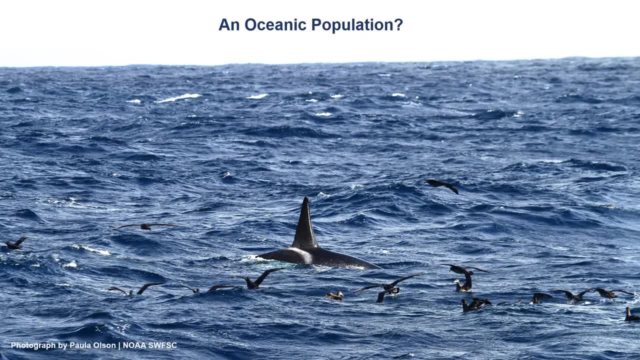 It was feeding on pygmy sperm whale, but all the encounters that we've had have been with them eating marine mammals, and most of this work has been done by NOAA Southwest Fishery Science Center, who we collaborate with. who we collaborate with, And you can see these- there's albatrosses out here that we're feeding on the carcass, but we really don't know where these animals fit in. 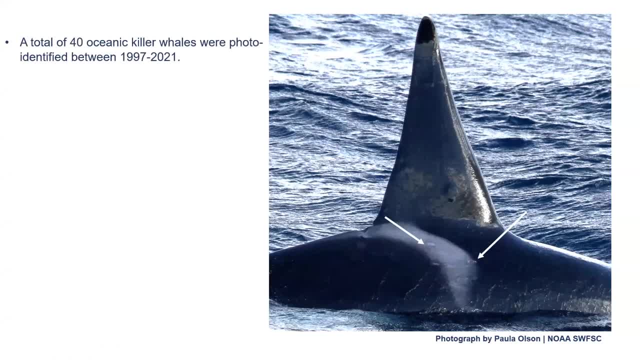 So here's an animal, a large male, here, And it was. we've had a total of 40, and we have a total of 40 of these animals identified between 1997 and 2021 through data we've either had from encounters or through consolidation and collection. 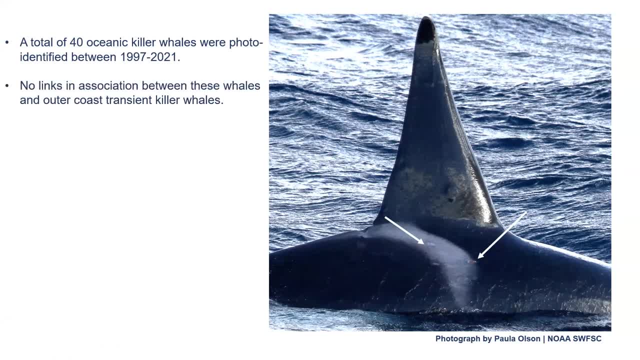 We have no links between them and known outer coast transients or any killer whales that we know of, found predominantly seaward of the continental shelf, so far offshore. And we have no links between them and known outer coast transients or any killer whales that we know of, found predominantly seaward of the continental shelf, so far offshore. 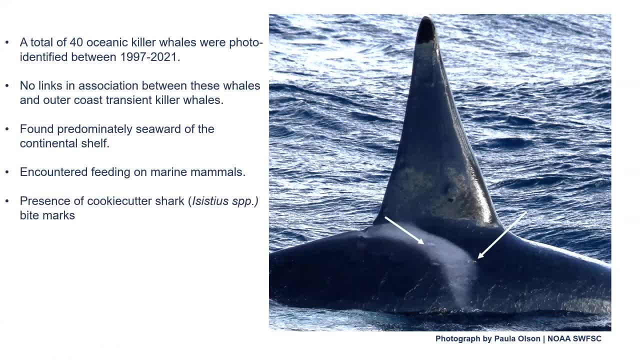 Encountered, feeding on marine mammals similar to transients. Also, they had this unique thing called the presence of cookie cutter sharks And, as you can see here on the saddle patch right here, you can see these bite marks. Some of them are older, more white. 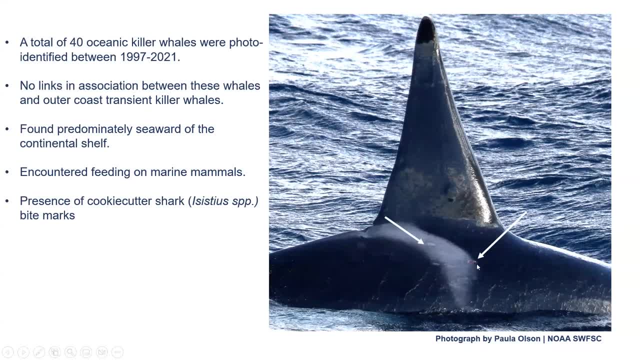 Some of them are black, but there's fresh ones to where the adipose tissue or the epidermal skin has been broken, and you can see the actual pink tissue here- And these are caused by the shark species called a cookie cutter shark, And what's unique about this is that these marks are only found on animals that spend time in offshore waters. 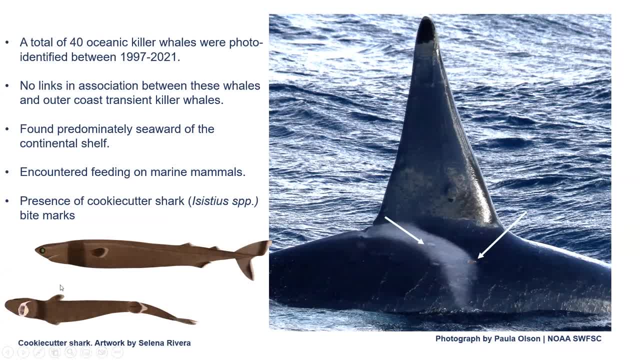 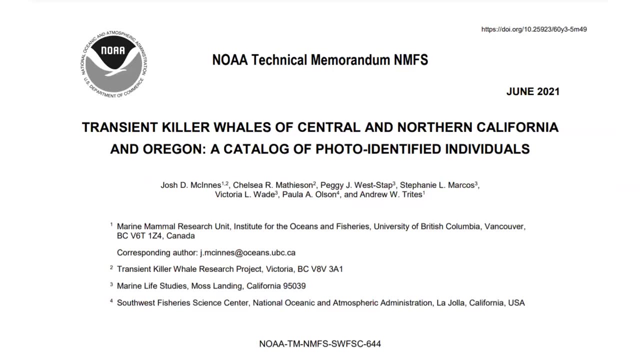 These sharks in general are deep water pelagic species that only feed in warm offshore waters, So it really shows a little bit of an indirect presence of these animals and far open ocean habitats. So the end of this will be published in 2021, a new catalog for transient killer whales off the seashore. 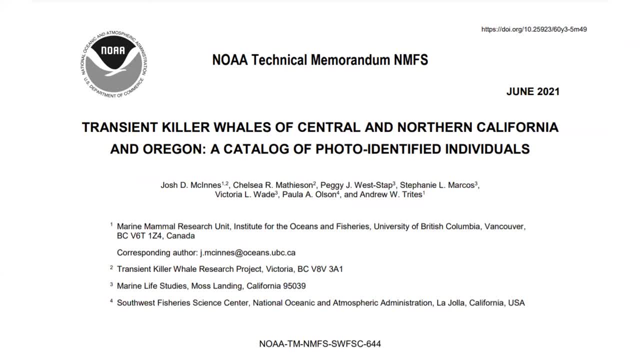 It's going to be released on the website. It has all the individuals that we photo identified throughout that entire study. We were very happy about this. We'll be updating it every couple of years and we're going to especially as we start to learn more about killer whales off Oregon and California. 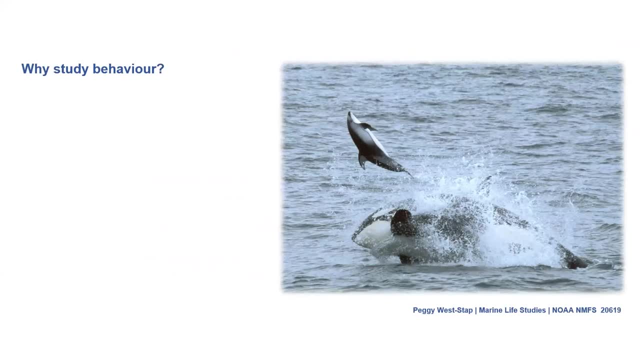 So one of our main. the third thing I would like to talk about is our behavior study. This is kind of where I focus. a lot of my attention is animal behavior. So why study behavior? Well, animal behavior lets us understand how animals interact with their environment as well as each other, how top predators such as killer whales may influence their habitat. 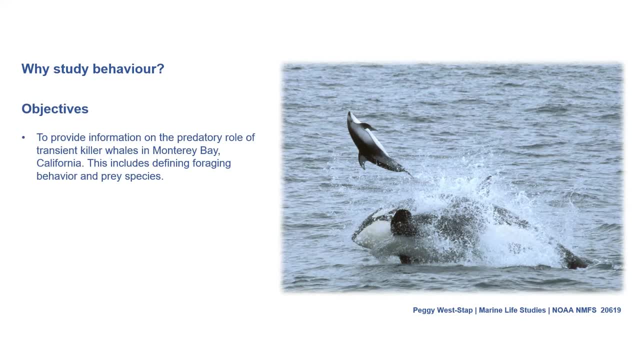 And some of our objectives were to provide information on the predatory role of transient killer whales in Monterey Bay, California, but we're also extending this to the Oregon coast, And this includes defining their behavior as well as the type of prey that they're eating. 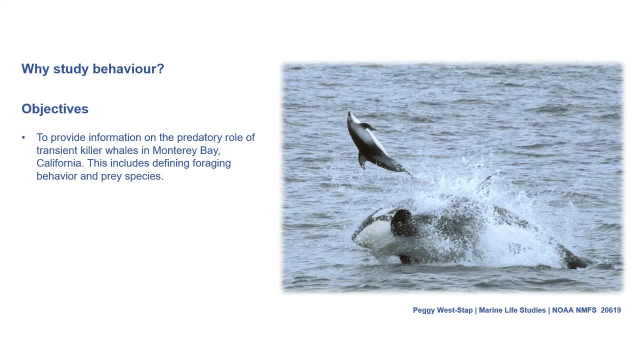 And this is getting more and more important, especially off the Oregon coast, with seals and sea lions which are interacting with fisheries. understanding how killer whales may be part of this ecosystem and how they may affect the prey populations is an important aspect and critical for understanding fisheries management. 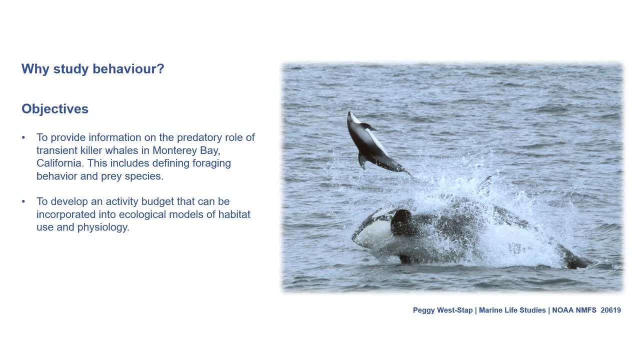 We also wanted to develop an activity budget. So an activity budget is a behavioral budget where we look at what killer whales are doing, what kind of behavior, what kind of percentages of each behavior are being used by these animals. It can help with development. 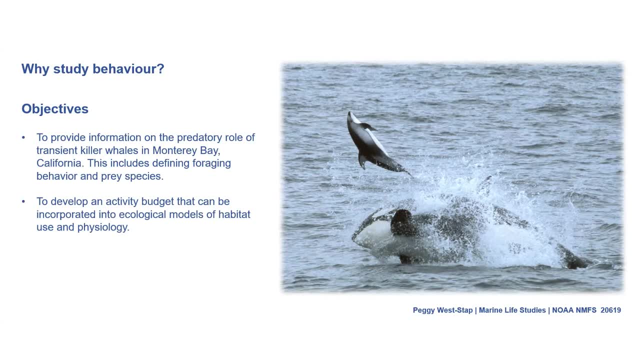 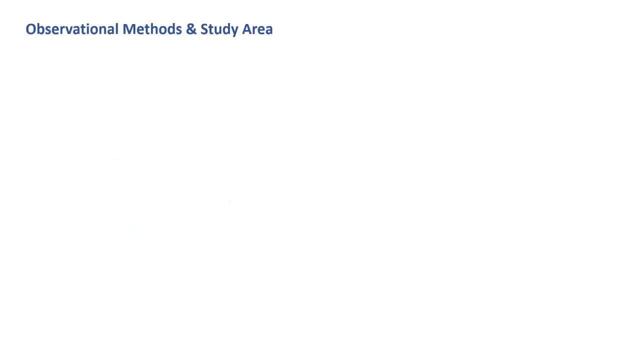 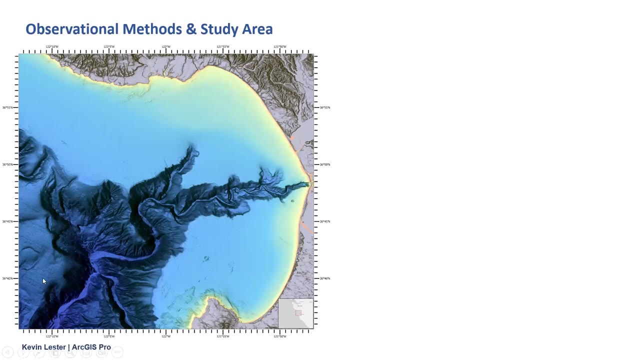 We also wanted to develop an ecological models for understanding habitat, as well as physiology, which is like energetics, But we also want to provide information on seasonal occurrence, the types of prey and the habitat use patterns. So what do we do? We use observational methods. This is Monterey Bay here, a much more up close map, but the most distinguishing feature of the bay is this big canyon. 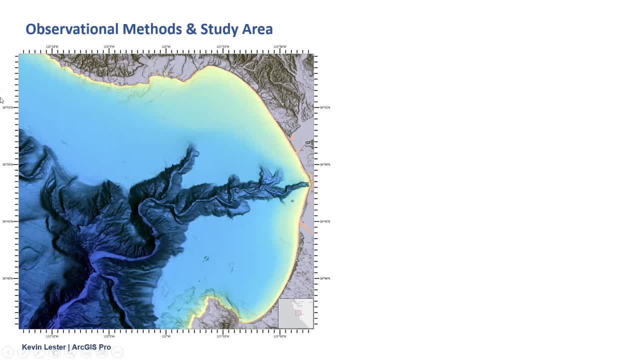 It comes all the way into shore. as I mentioned, this continental shelf narrows and comes right in, and this is the submarine canyon We used. Once again, we used opportunistic encounters, the NOAA fisheries science surveys, as well as whale watching to try to help get sightings. 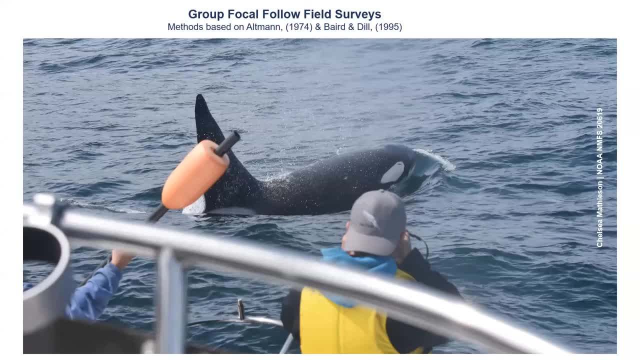 But one of the big methodologies we used was focal follows. A focal follow is where you're constantly following an animal or a group of animals and you're collecting behavioral data systematically. So you're collecting information on a time basis where, say, every five minutes, you take a location of where that animal is seen what it was doing. 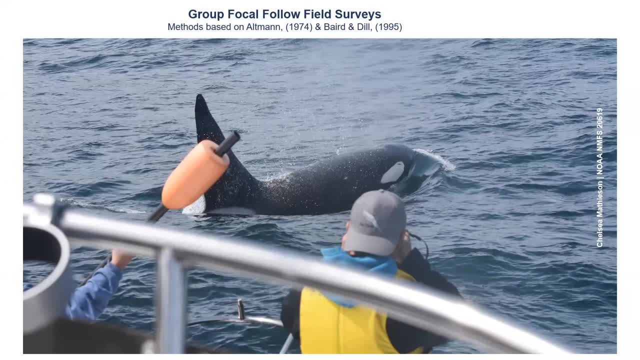 and what the group was doing, And we did this for this population. Every few minutes would take a location, using a GIS, using latitude, longitude, as well as identification of the animals and what predominant behaviors. So if they were, how the distance between individuals, how long dives were the respirations, what they were feeding on, how far apart they were? 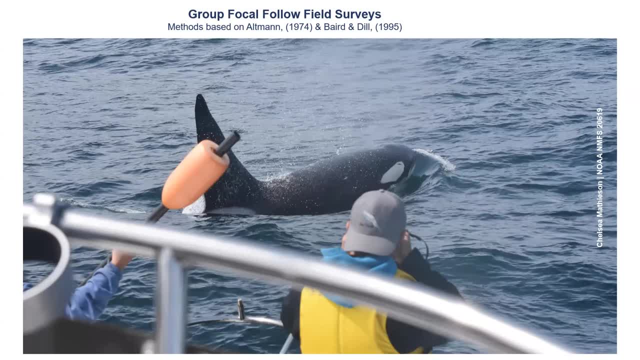 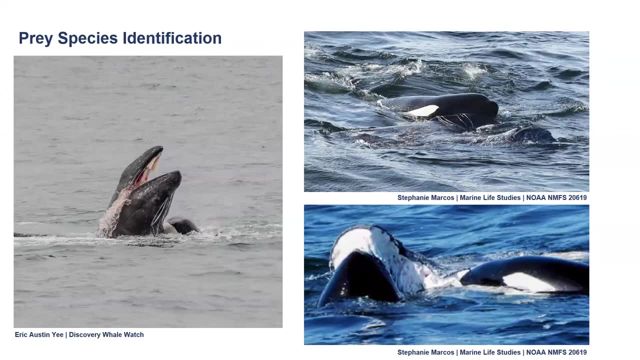 This was all important for defining specific activity, states or behaviors. This is kind of gruesome. This is the most gruesome photo you'll see, But this is. we also was important to identify prey, And this often involved being close up, And in California, especially off the outer coast of central California, we saw a lot of gray whale calf predations in the spring, in March and April, where the outer coast transients seemed to spend a lot of time. 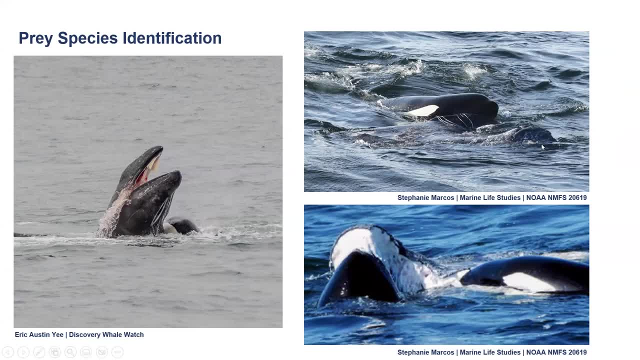 This is a photograph here of a gray whale calf being attacked. This is a carcass of a gray whale and often being able to define the amount of tissue and blubber in the water if there was birds present and how killer whales coordinate. 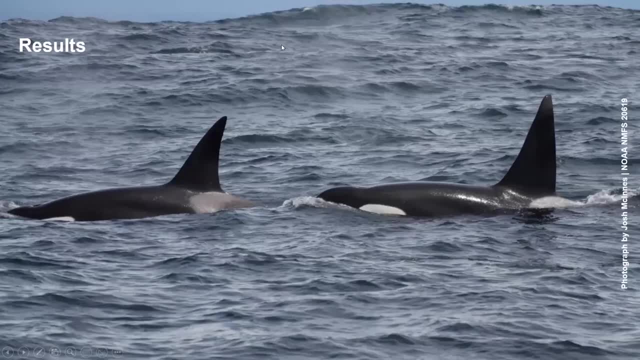 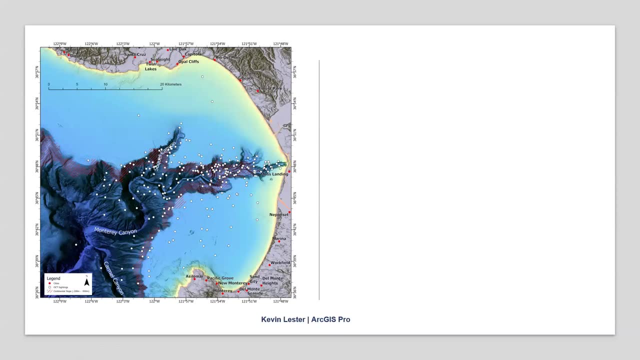 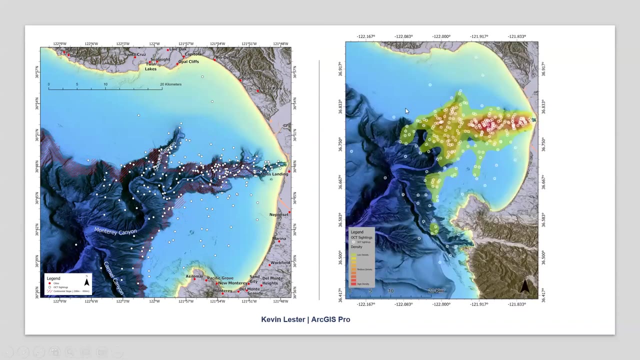 And how they share prey is also very important. Our results from this study- One we had close, we had over 260 encounters for this study, But 100 encounters, 260 sightings, 100 encounters with transient killer whales And this heat map- here you can see our colleague Kevin Lester- shows kind of where transient killer whales and our encounters were predominantly found, which is along this canyon area. 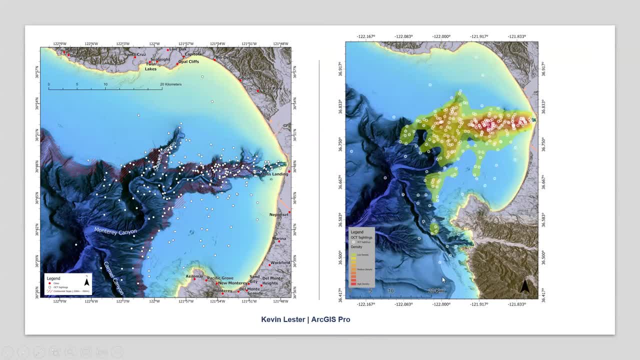 Where they seem to ambush grasslands And we can see the gray whales as they migrate up the coastline. So as gray whales head north from the warm lagoons in Mexico, they kind of hug this coast And then, as they cut across the bay, you'll see that they sometimes hug around here and they'll kind of cut like this and then kind of go up because they're heading north up to Oregon. 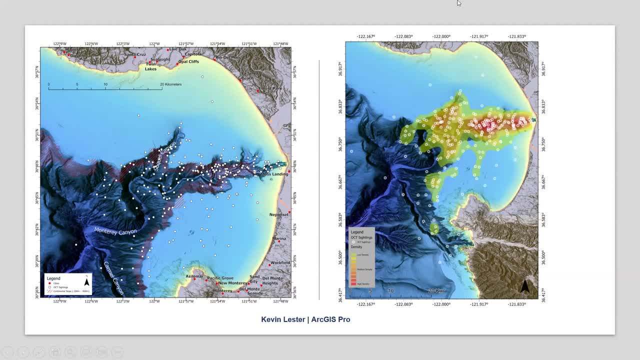 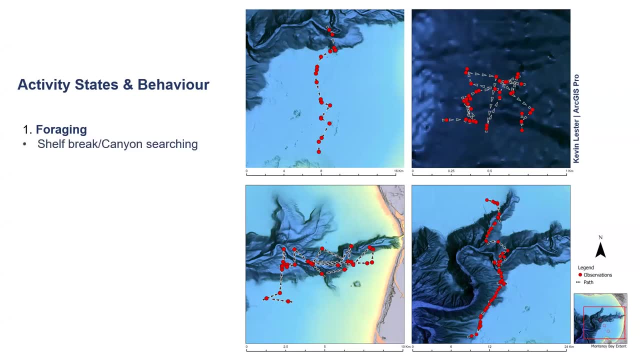 We're starting to learn, though, gray whales might also be being killed off the Oregon coast. It's something that we're still investigating, But we just find activity states, So foraging was the number one activity state, And that involved a couple of different types of foraging. 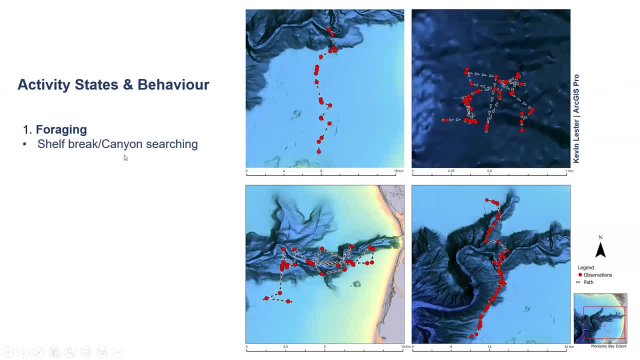 Or sub-behaviors, One being what we call shelf break slash canyon foraging, And that's right down here in this panel, Where killer whales follow the edge of the canyon, sometimes crossing it, searching for prey along areas where a lot of upwelling and nutrients are found. 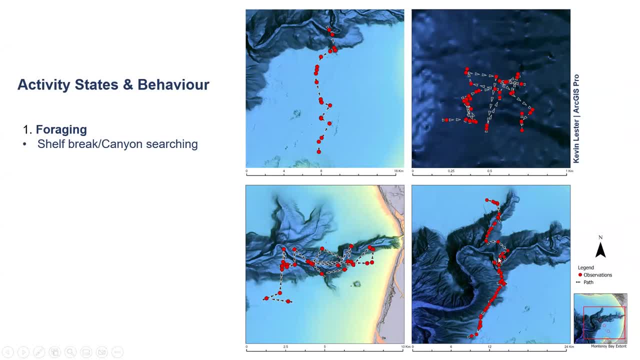 This is a brand new kind of behavior that has not been quantified before, So we actually came up with this term here. Also, open water foraging, which is on the other panel. here, which is different: Individual whales typically spread out over a kilometer. 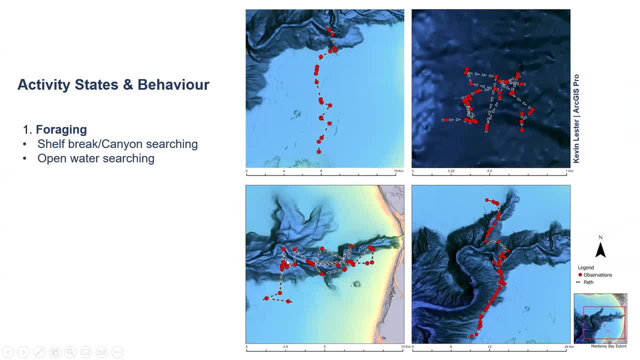 And often do this. zigzagging behavior- Where it's quite a long dive- five to six minute dives, where they zigzag all over the place A prey pursuit- is when they're actively actually attacking an animal. Feeding behavior- when they're feeding- that was also how long they fed- was important. 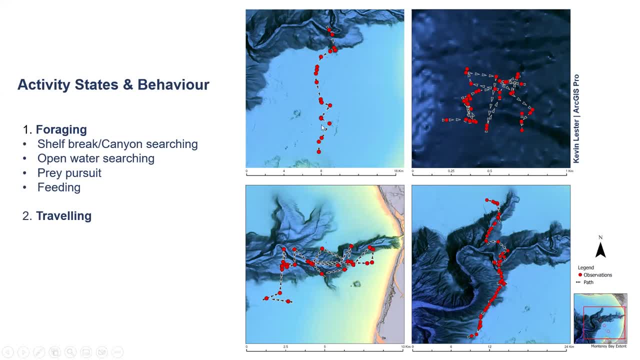 We also had traveling, which you can see up here is when they're actually cutting across an area in a linear direction And this is feeding up here where it's very stationary. So our ability to plot where we were was within 50 meters. 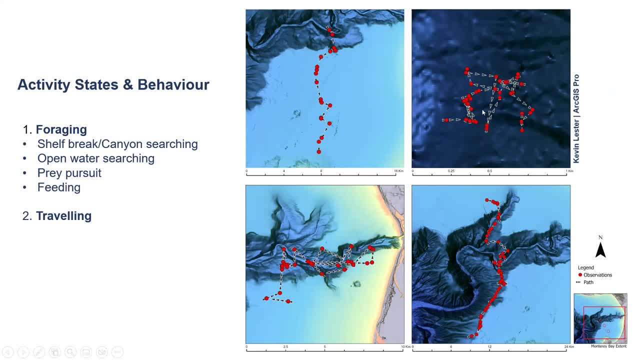 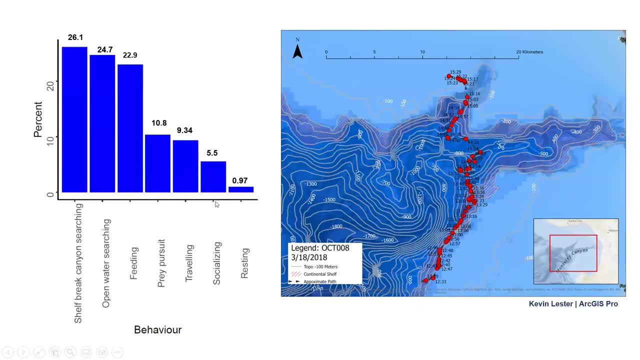 Of whales with our research vessel So we can kind of see their movements, was similar to where our boat track was. And then we also had socializing as well as resting. But you can see the percentages here of the different kinds of behavior. 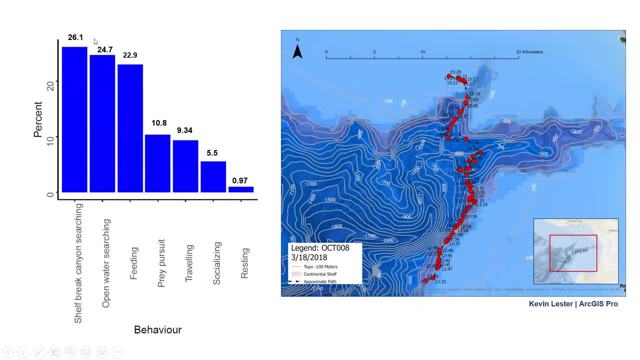 One shelf break searching, which I said that canyon searching was. 26.1% of the time in Monterey was spent utilizing this behavior, 24.7%. for open water searching And then resting was one of the least behaviors And this behavior was then compared to others. 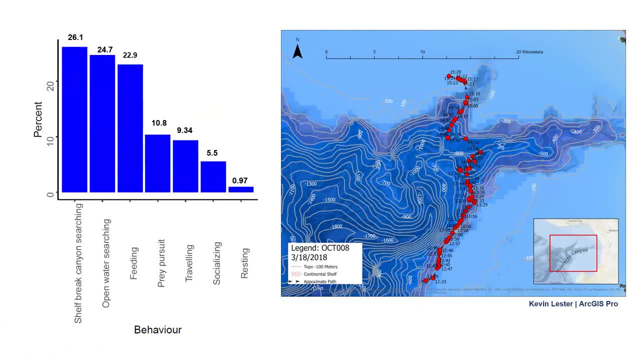 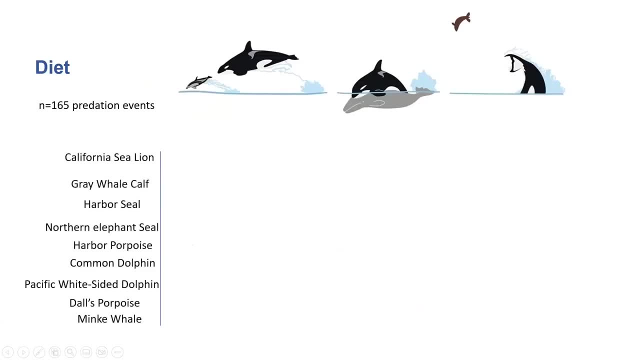 So we did a lot of research through activity budgets that have been formed for transients, And we found a very similar trend, And these results from this are currently publishing. Our diet consisted of the predominant California sea lion and gray whale calves, But in the spring this was what we saw. 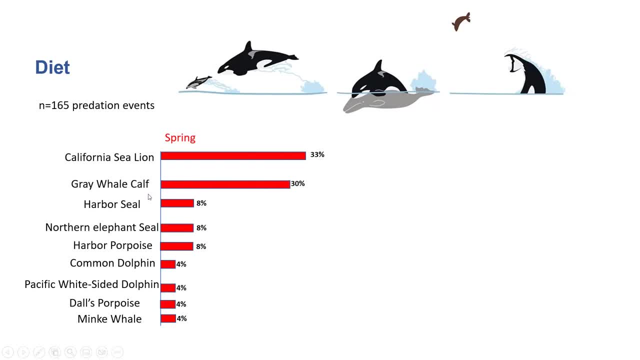 33% was California sea lion, 30% was gray whale calf And then less than 10% were a number of other species from harbor seal, northern elephant seal down to minke whale. We see California sea lion dominated. Gray whale calves are already, during the summer, fall and winter, either up in the feeding grounds in the Bering Sea or off Oregon or the Pacific feeding group population. 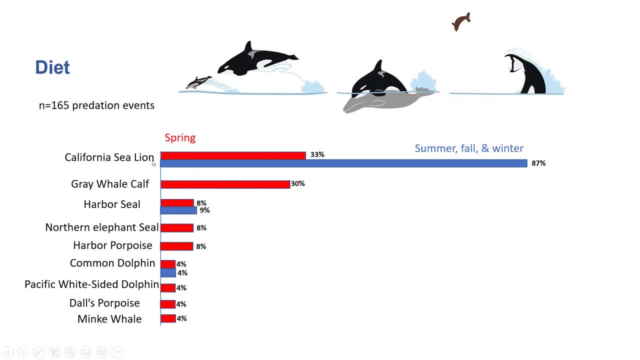 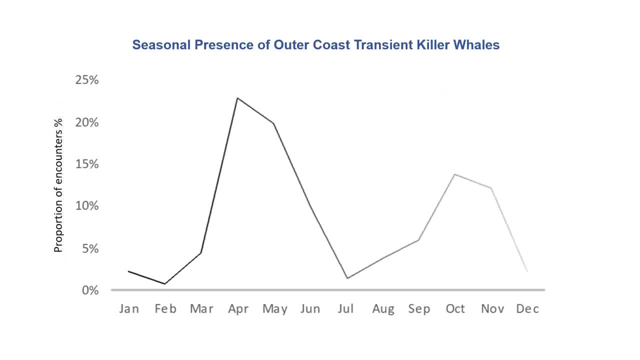 Or they're making their way back down the coast. But we don't have any predation events for gray whale calves outside that period. Seasonality for transients was bimodally distributed, So similar to Oregon. in California we see kind of a large spike in sightings in April and May and June. 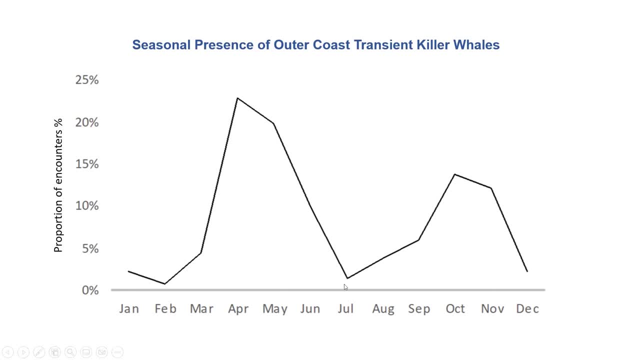 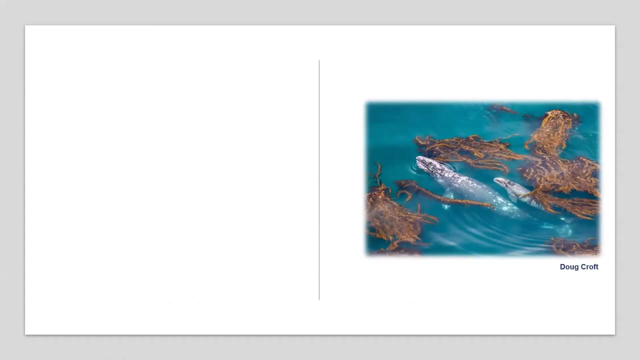 And then less in July, as we believe the killer whales may follow gray whales north And you can see here kind of in fall. So to really dive into this relationship of killer whale- gray whales, we had to really understand the ecology of both and a bit about the numbers of each that were happening. 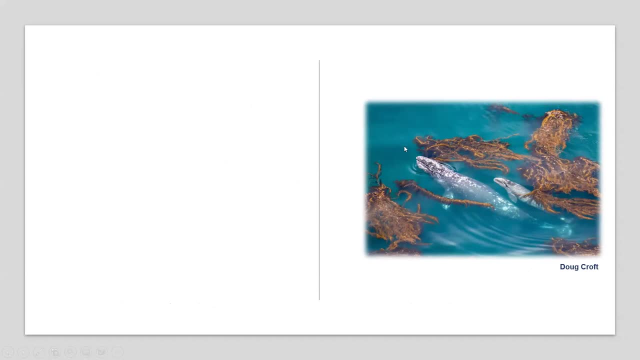 So gray whales, as I mentioned, this is off Big Sur, California. They migrate up the coast in the springtime, Calves are born in the lagoons, the tropical lagoons, And they go north with their mother in April and May. 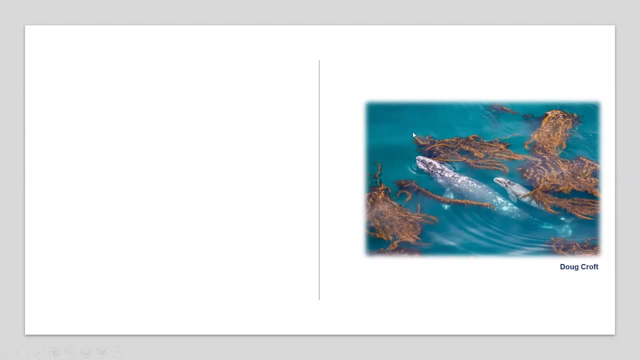 So, as they head up the coast, though, their NOAA Southwest Fishery Science Center actually conducts a census for gray whale calves off Point Pedras Blanca, which is a light station, And they count the calves, And it's only about 100 kilometers south of Monterey, California. 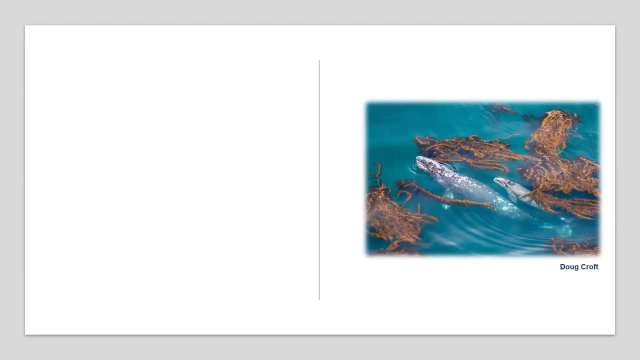 So we were able to take this data that they contributed to this study and apply it to some of the results that we have. And you can kind of see here- this is a gray whale- calf count is the orange, So the number of calves 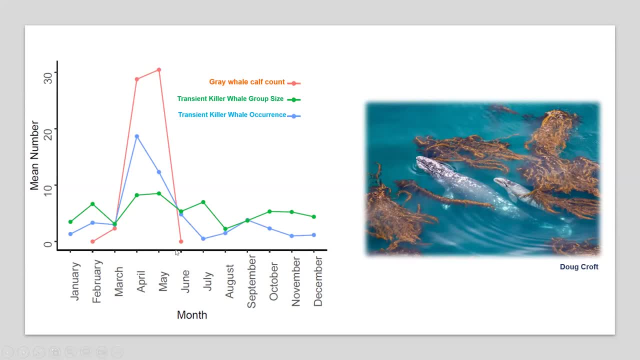 And calves are only counted between March and May And there's zero counts because by that time the calves are already headed north. So this is kind of that spike. But transient killer whale group size you can see here also kind of spiked for the number of transient killer whales that were seen, the number of groups that were seen, but also the occurrence of transient killer whales. 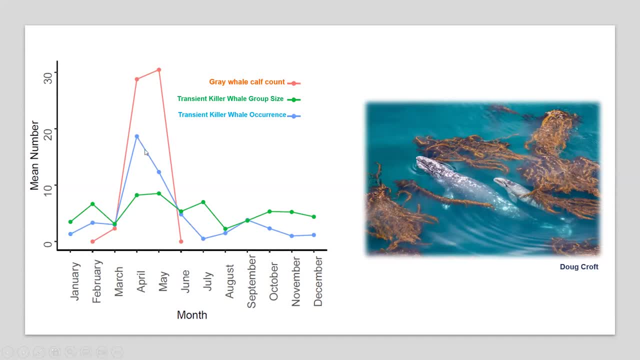 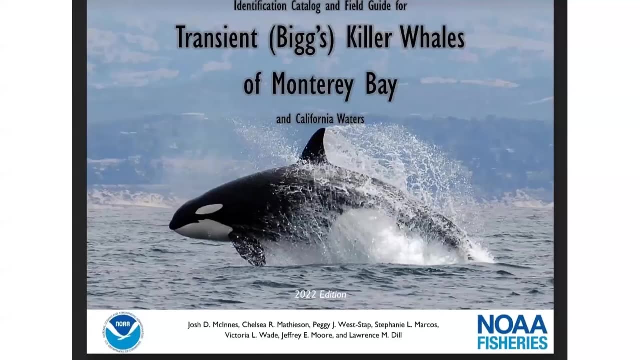 What you can see here, that occurrence is the number of times killer whales were seen, And you can see a similar spike, And this was also statistically significant in our study. Finally, we're stoked to have a brand new publication coming out in 2022 dedicated to transient killer whales. 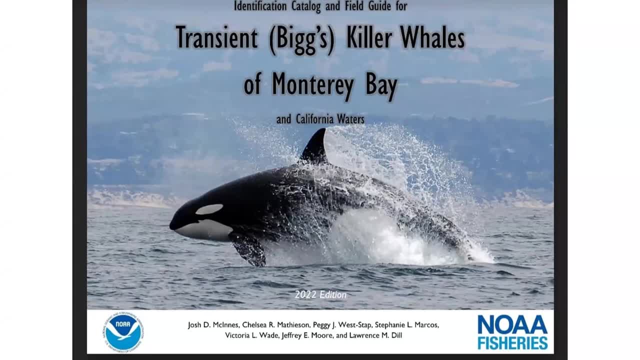 It's a field guide for naturalists and people that are just interested in killer whales. It's non-technical, It's more of a natural history guide that's produced by NOAA Southwest Fisheries Science Center for California And we're currently in the process of building one for Oregon as well. 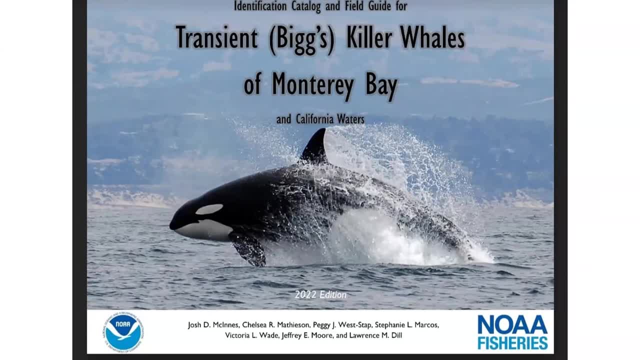 So this will be available online for free And we'll have an Oregon one hopefully up in the next year or two. I'm currently writing, So it's pretty exciting because we're, as I mentioned, with the increase in our Oregon efforts and with the amazing community in Oregon, we're learning so much more about killer whales. 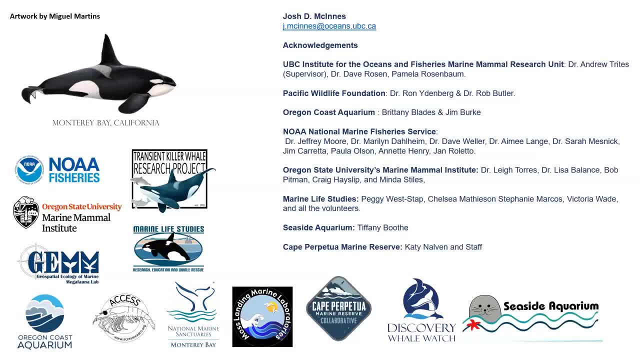 I just would like to acknowledge. there's so many people that I'd like to acknowledge the entire Oregon community. You guys are all so amazing. This wouldn't be possible without the multiple people that are out there providing photographs and sharing, as well as organizations like the Cape Perpetual Marine Corps. 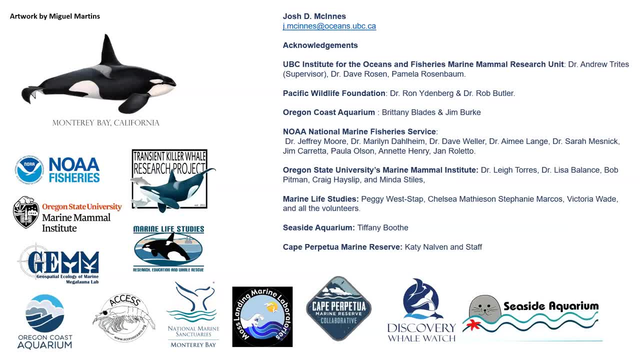 Organizations like the Cape Perpetual Marine Reserve, as well as Oregon Coast Aquarium, Seaside Aquarium, NOAA Fisheries, as well as Oregon State University, who we collaborate with quite a bit, And in California, that wouldn't be possible without the National Marine Sanctuary's marine life studies, as well as Moss Landing Marine Laboratories and Discovery Whale Watch. 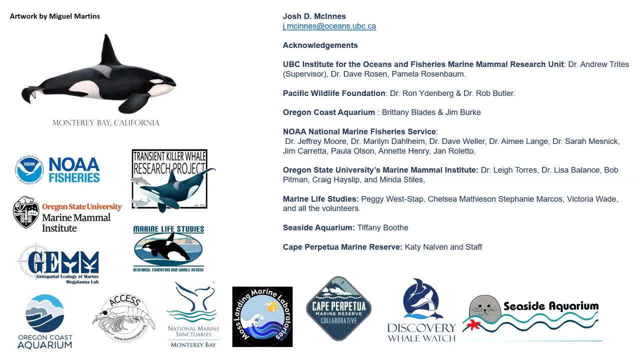 But I just want to thank the Cape Perpetual for letting me speak today And it was awesome talking to everybody. Thank you. 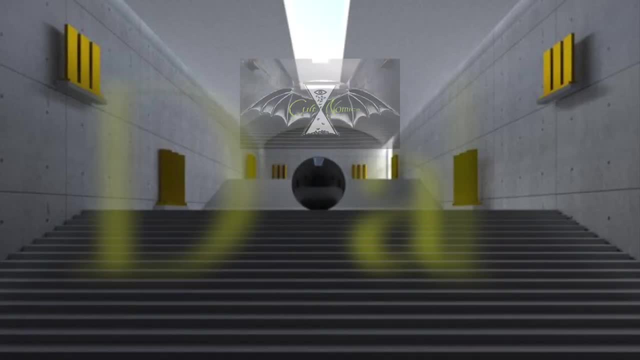 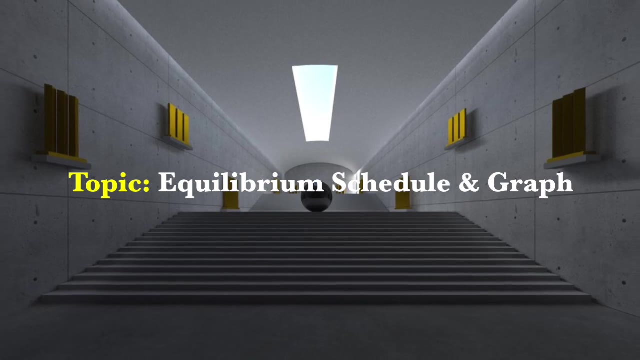 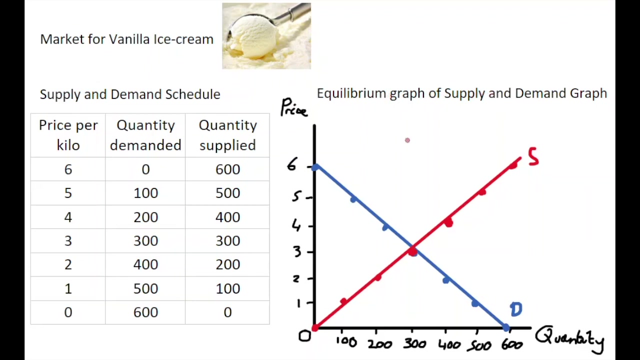 Hi, guys, and welcome to Cultnomics. My name is Paul Henley and today I'm going to be chatting to you about a demand and supply equilibrium schedule and graph. Okay, guys, so in this video we're going to look at deriving equilibrium supply and demand on a graph. We're going to take the 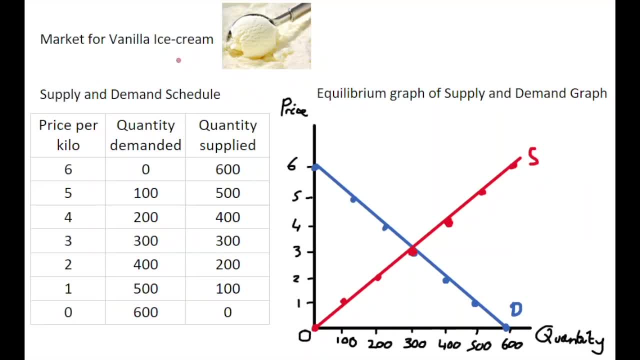 market for vanilla ice cream, which is quite the generic market, with lots of buyers and sellers, none of which dictate price. and what we have over on the left hand side here is the supply and demand schedule. This is a table of figures that have the price of their product, the quantity, 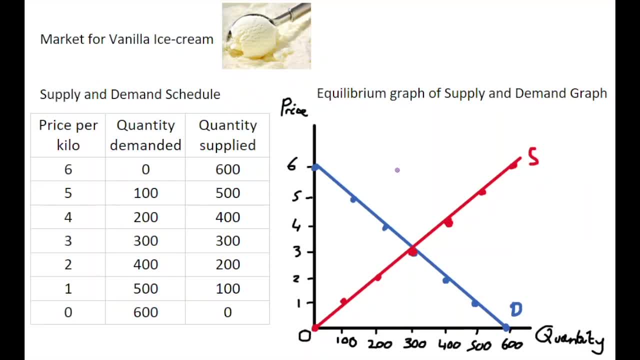 demanded and quantity supplied. Over on the right hand side we have our equilibrium graph, where we've taken these demand schedule figures, as we've shown in previous videos, and mapped them out to give us both a demand curve and the supply curve. So, in order to determine the equilibrium point on 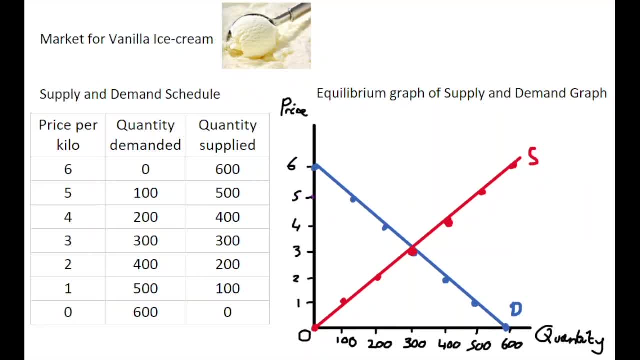 this graph. here we're going to need to have a supply and demand graph. So, in order to determine the equilibrium point on this graph here, we're going to need to have a supply and demand graph. What we're going to do is we're going to start off at a higher price level than equilibrium. 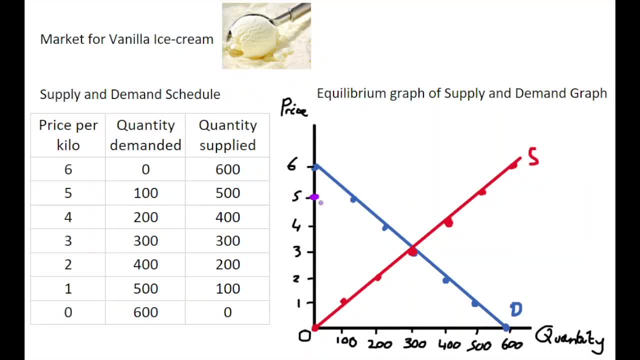 So we're going to start off here and assume that we've dropped into a market at one point in time. The price of vanilla per kilo is 5 and we can bring that price straight across to where it hits both our demand and our supply curve.